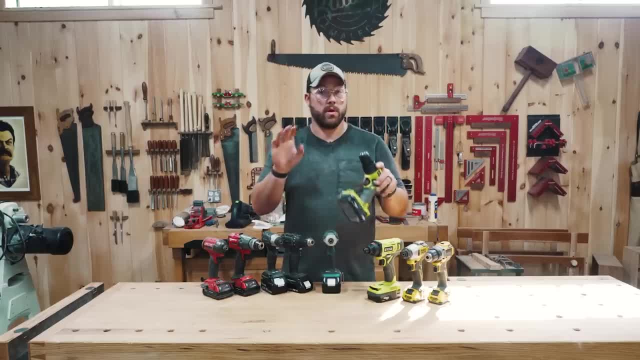 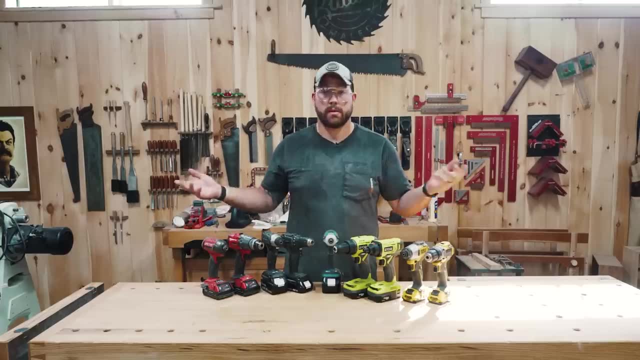 looking to get into cordless tools, definitely want to check them out. 18 volt if you can afford it, And I would definitely suggest your first set of drills being in 18 volts, because more power the better right. You never want to not have enough power when you can have more. 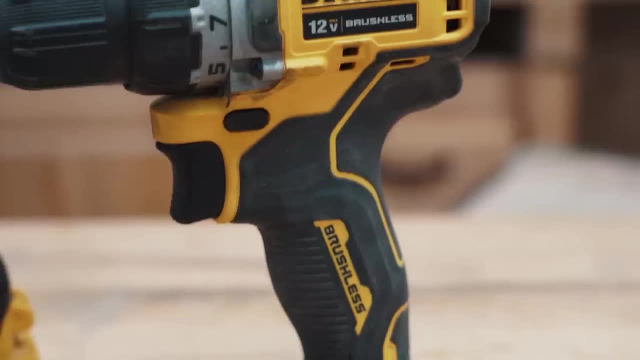 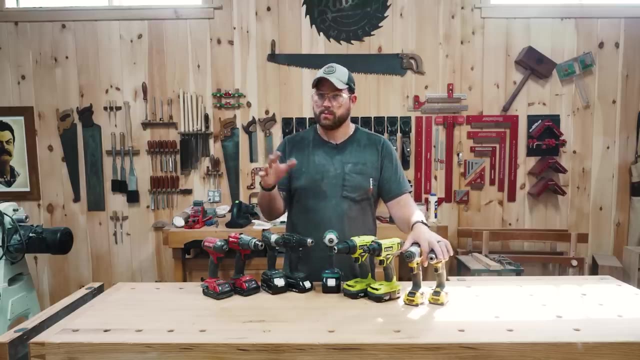 but there are options out there for less. We've got these 12 volts here. We love these. We use them a ton since they showed up. They're compact, They pack plenty of punch for small things. but we can't do any of the. we can't fasten into walls, We can't set studs, We can't. 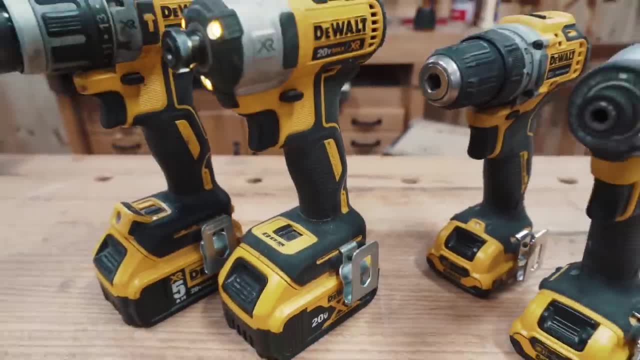 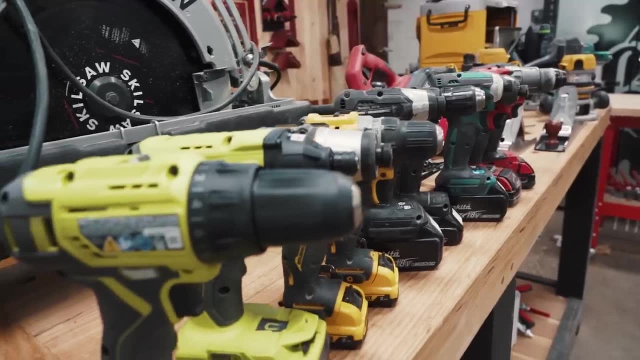 do any of that bigger stuff with them, because they just don't have the beef. There's tons of brands out there, tons of options out there. We love any of them pretty much. We use, you know, DeWalt Daily, Makita Daily, Milwaukee Daily, And you've seen a lot of these in our content. 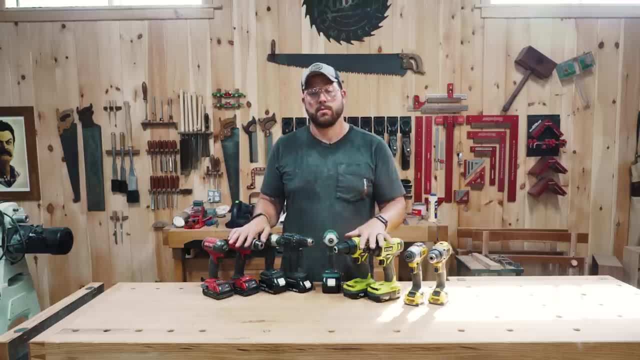 because they're all really, really good. But if you're looking to get into them yourself, consider the battery platform you want to be on long-term and buy that first Impact driver, the first thing you should buy, whether you're in the woodshop workshop or a. 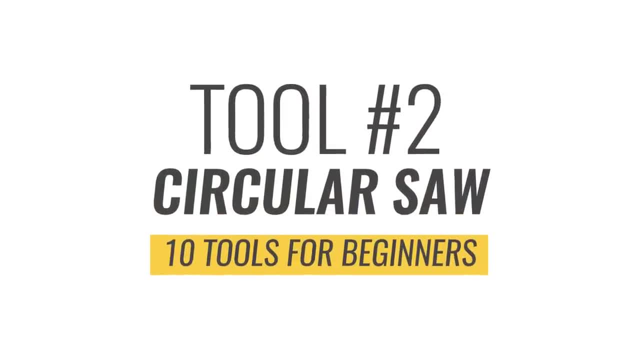 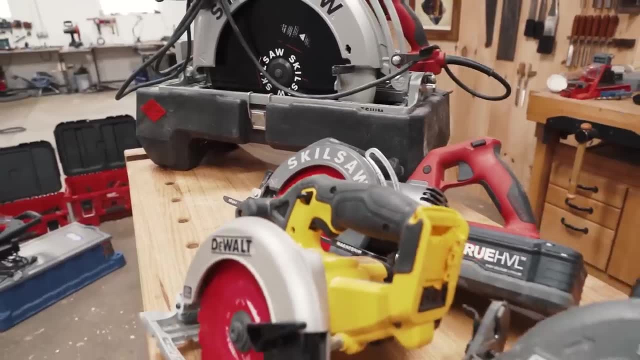 homeowner, in my opinion, All right. So the number two tool you're going to want as a beginner workshop or the home in my suggestion, is a circular saw. There's tons of options out there. You've got the, you know, seven and a quarter standard sidewinder saw which is going to look. 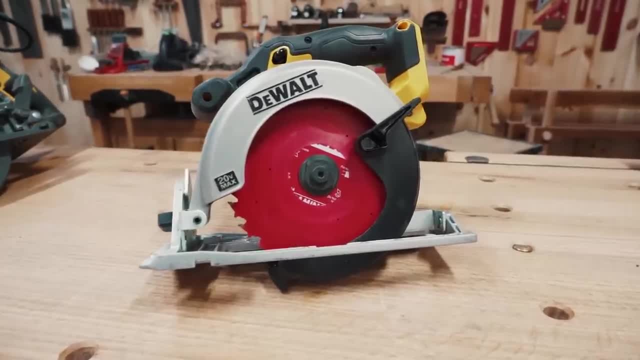 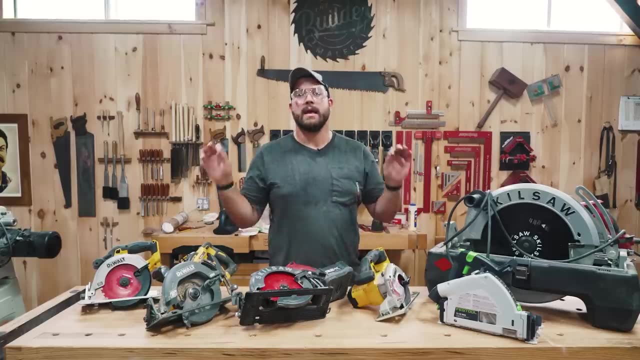 like this. This is not a seven and a quarter, but you get the look. You're going to have your rear-handled worm-driven saws that look like this, corded in battery powered. tons of options out there. Get whatever you can afford. I suggest a seven and a quarter. 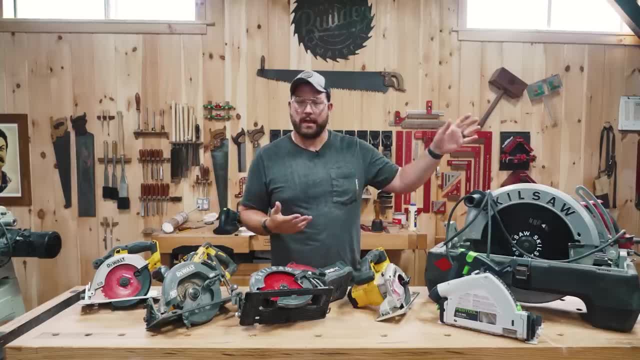 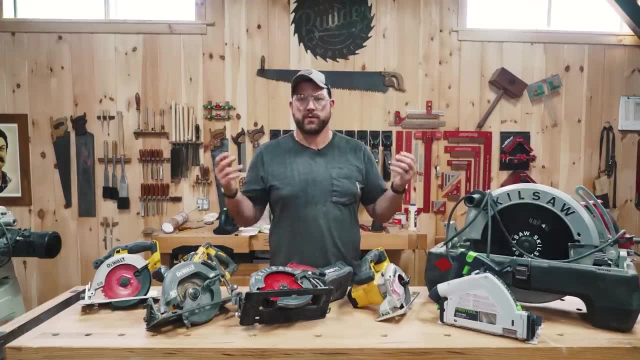 inch, saw that plugs in the wall. I've got a DeWalt one. Ironically I left it at the house that I've had for about 10 years now. It just stays at the house because it's always there to use And it works phenomenally. You can use it with a straight edge. You can do some really. 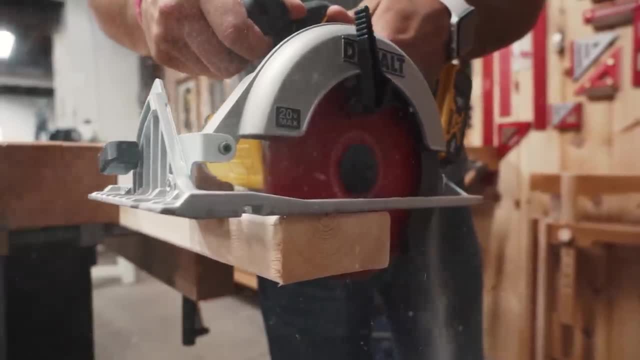 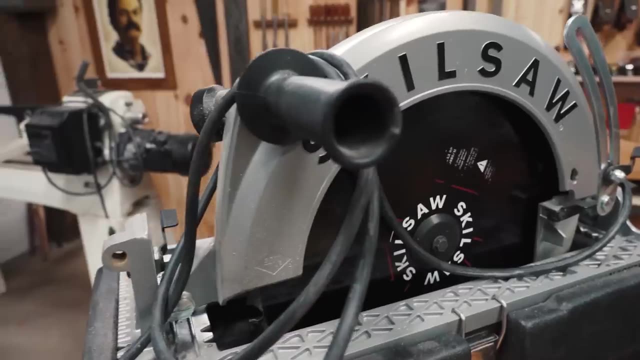 precise stuff, And they are like one of the most versatile tools to have in a shop, Whether you're framing, whether you're building furniture, whether you're going over to your buddy's house to chop up, and they're great to have. Now, a couple of things you're going to want to consider are the battery. 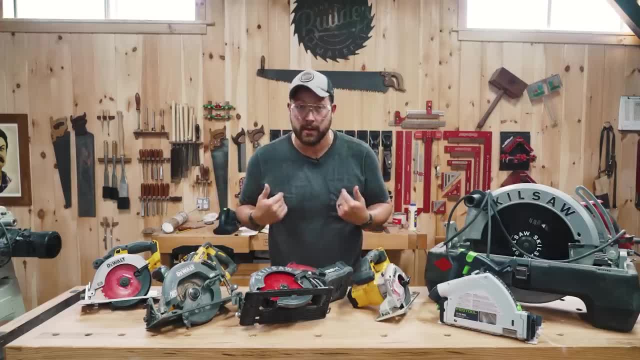 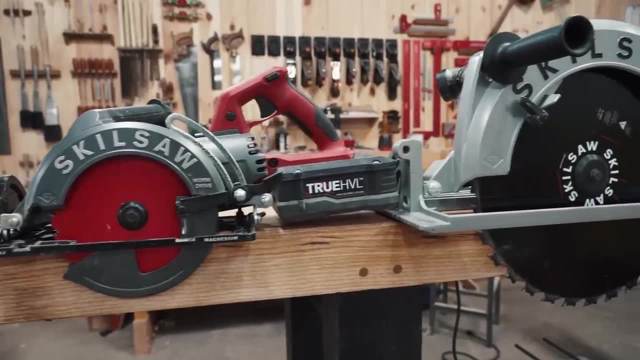 platform you own because you just bought a Drill and Impact, because you're listening to me, If you're going cordless, is it in the same battery platform? That's important. Also, the size of the saw. If you're going to be cutting tabletops and stuff, go with the seven and a. 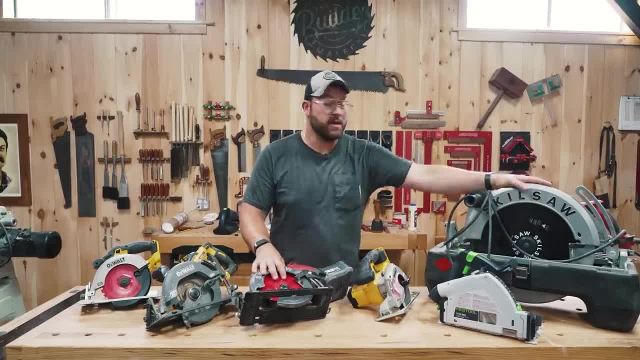 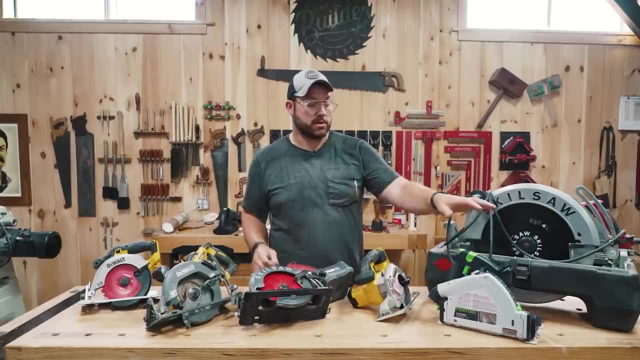 quarter inch. Gillsaw here makes a 10 inch. They also make this 16 inch beam saw. They've got monsters When you get used to using this in your workflow. the next evolution is going to be the track saw. A bunch of brands have them. You guys have seen a lot of them. They're going to be. 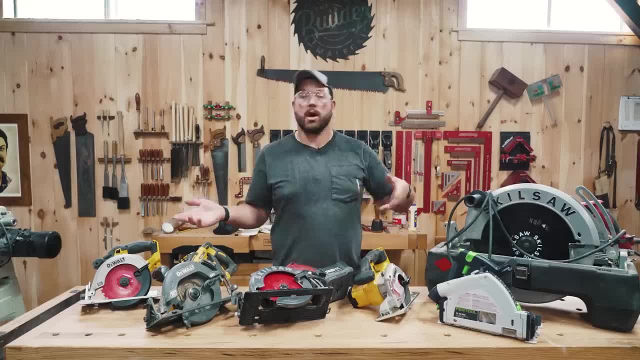 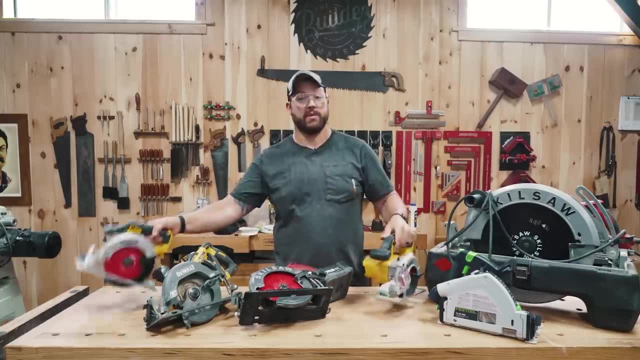 in my content and they also work amazingly. The last thing is going smaller If you're doing stuff that say you're on a ladder or you need to be really mobile. they've got five and three quarter inch. They've got six and a half inches. out there Tons of options, but we recommend the seven and a. 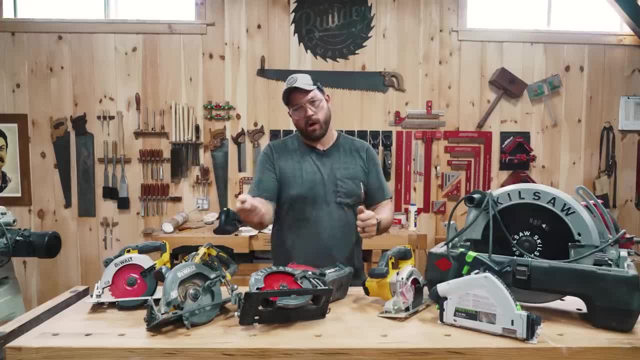 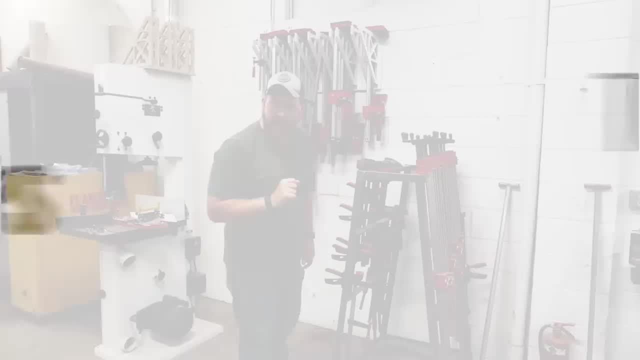 quarter inch regular sidewinder plug in the wall, circular saw Going to be the number two tool that you should have. All right, the number three tool that I suggest for all beginners is going to be the clamp, Hence why we're in clamping. 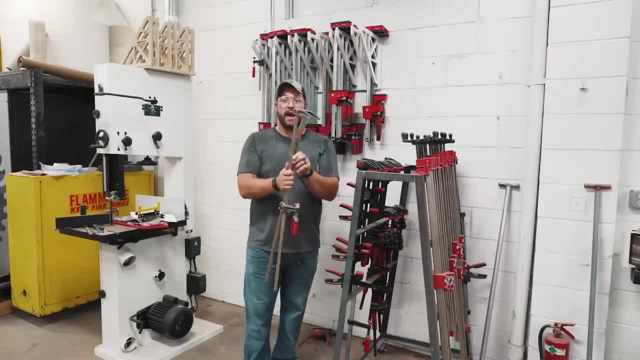 These are literally the first two clamps I ever purchased. This is called an F style clamp, As you can see- I don't know which way this comes up on camera, but it looks like the letter F- Highly versatile, very, very, very popular and very affordable. These basically get the job done. 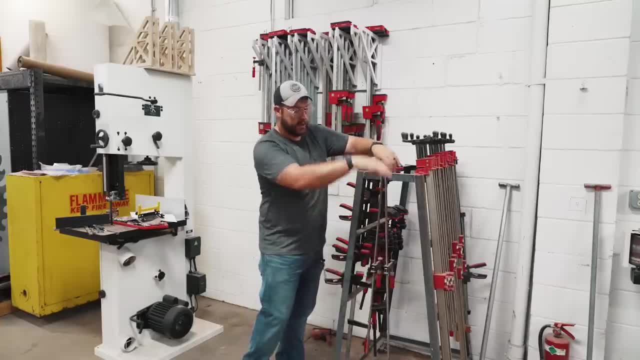 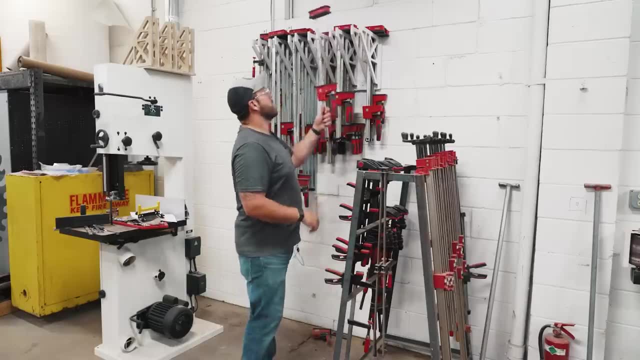 Now are they the best? No, but if you're getting into it, you definitely want to look into them Now. there's a ton of options out there to go with these, and you see them in my content a lot. One of the most popular is going to be what's called a parallel. 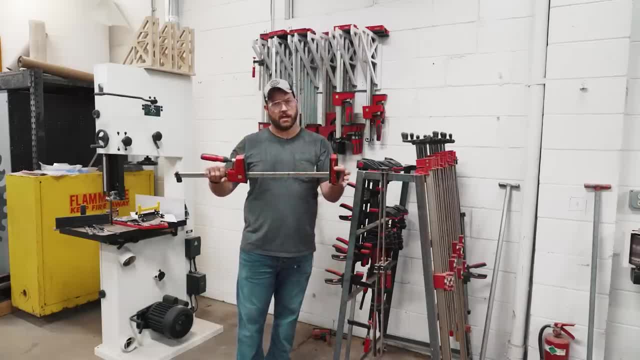 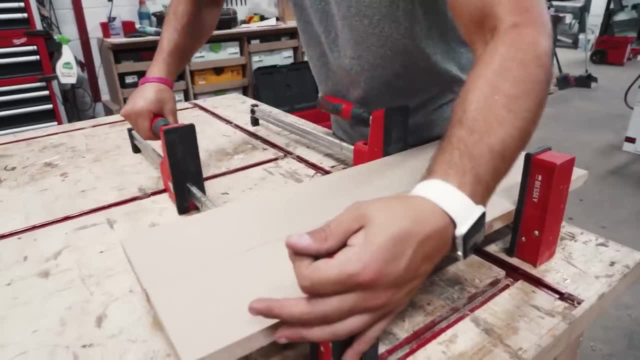 clamp. These are going to be the most expensive option, most likely in most cases, but they are very specific to woodworking and they also do a very, very good job. They give what's called parallel clamping pressure and help panel glue ups a ton. They were one of the first upgrades that I 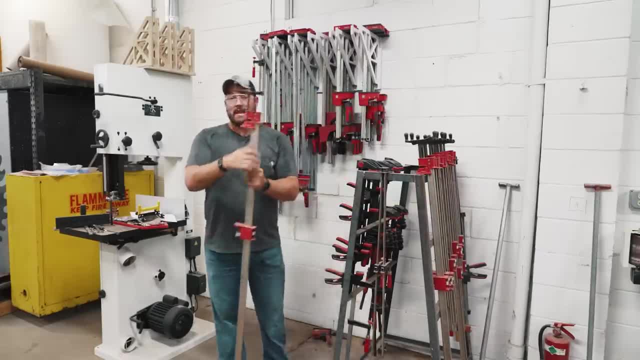 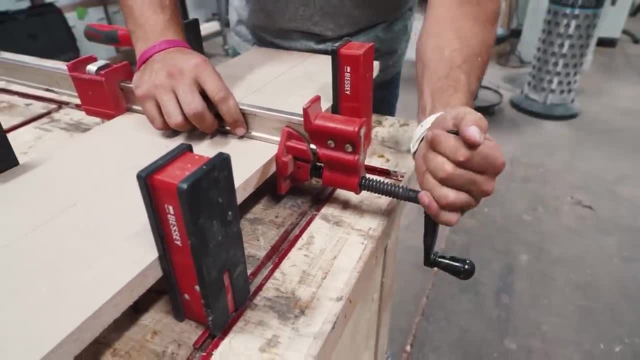 chose to get into when I bought more clamps after the first clamp. These are kind of a newer innovation and these are a step up from what's called a pipe clamp. These are an I-beam clamp made by Bessie. As you guys know, Bessie is a sponsor of ours and that's why we're going to be. 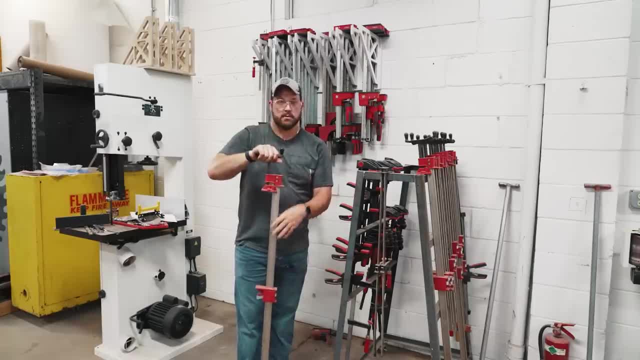 talking a lot more about that in a little bit. So we're going to be talking a little bit more about how you see a lot of red clamps from me, but any of the brands are pretty decent. Bessie makes the best and then everything else after, but you can get the job done with pretty much anything. 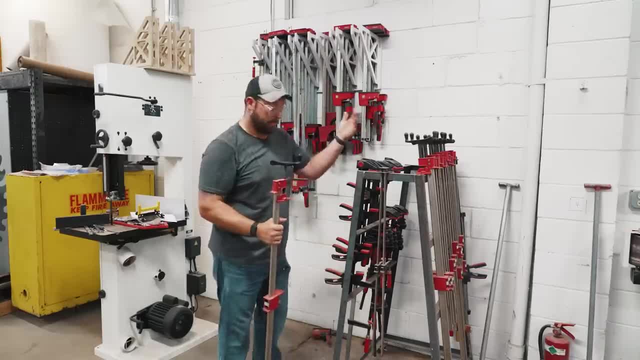 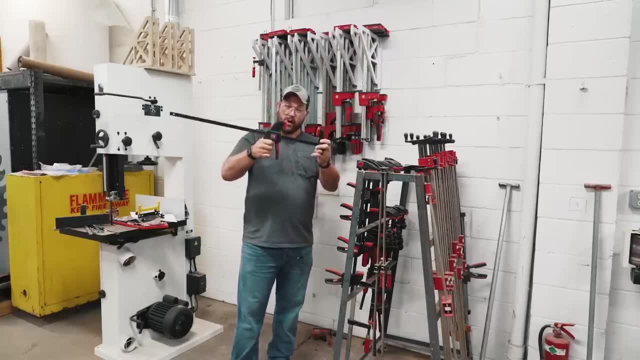 These are going to be able to apply a lot more clamping pressure, as is a pipe clamp. The third most common clamp you're going to see in my shop is going to be the squeeze clamp, and this is a squeeze clamp. Pretty much use it with one hand. We use them for a lot of things, mostly just quick. 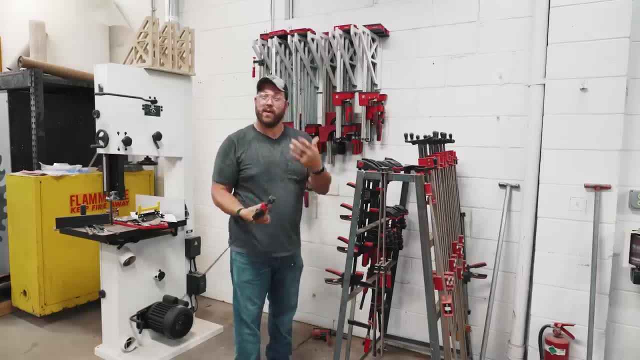 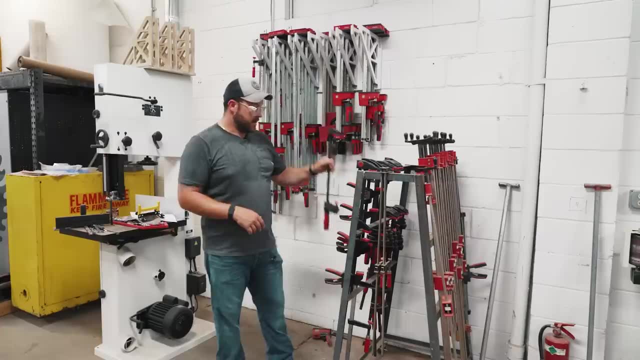 kind of clamp ups. We do not glue up panels with these, because even though they do have great clamping pressure, they don't work as well Once you start to get a bunch of clamps. they're really nice to have. And then Bessie also makes. 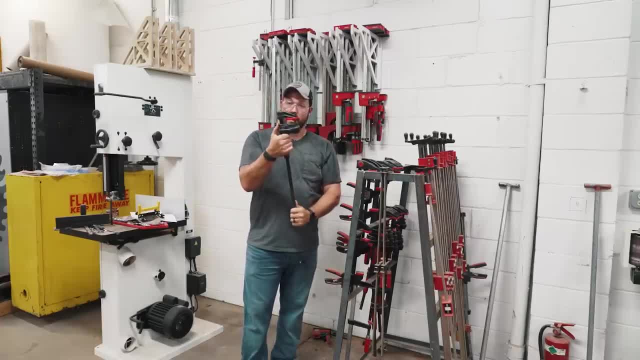 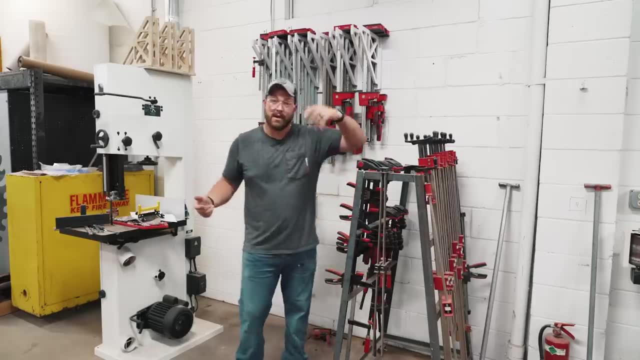 these single-handed geared clamps that you only need to use one hand to adjust and to tighten- Also another phenomenal option. but as you get up there in convenience, you get up there in price, and not all of them are a necessity. So number two option for all of Jens, in my opinion. 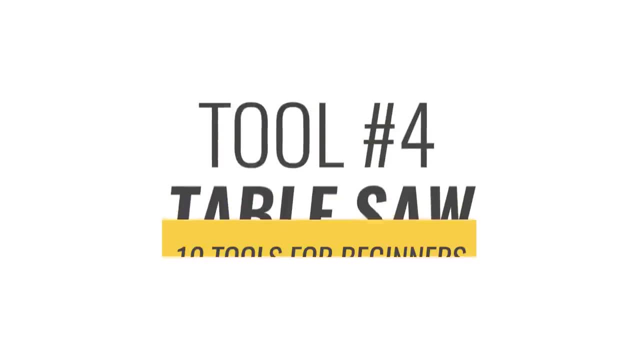 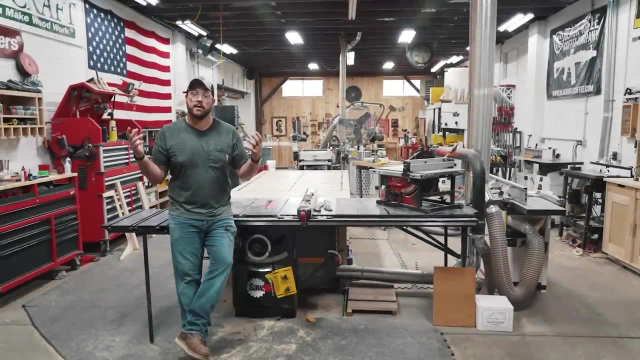 in a wood shop at least, is going to be the clamps. All right, Jens. the number four tool that I suggest for a beginner wood shop or workshop, or what do you call it, Whatever is a table saw. Here is my table saw, but this wasn't the first saw I owned. 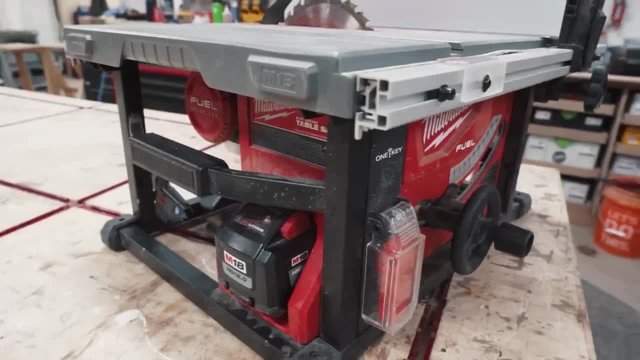 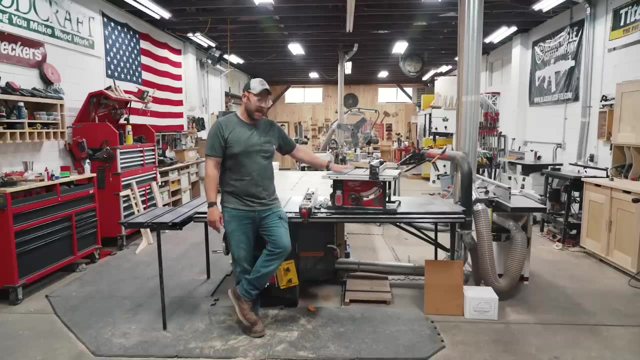 What I worked on first was it's called a job site saw, And you guys have probably seen this in some of my home remodeling projects. This is our cordless job site saw. This runs with- I think it's- a 10-inch saw. It's got a little blade in there and this one just happens to be. 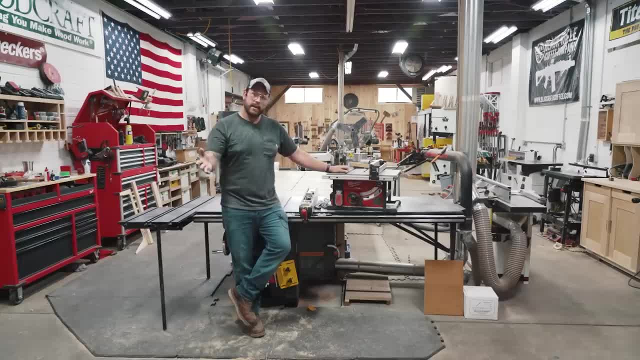 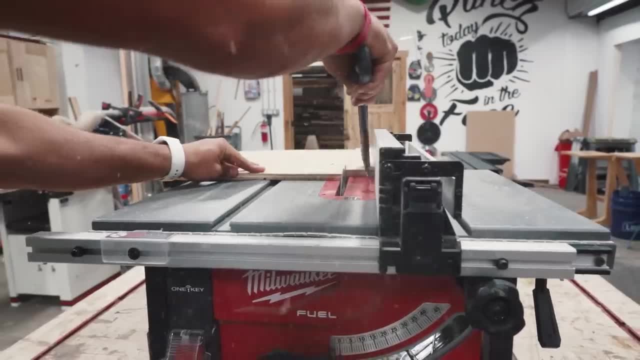 cordless. I have a corded DeWalt one as well. Brand doesn't really matter. The concept is it's small, it's lightweight, it's portable and it's easy- Easy to use and also pretty affordable to get into. I suggest getting into the table saw. 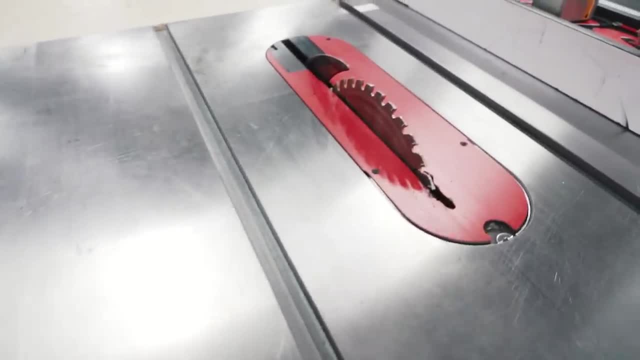 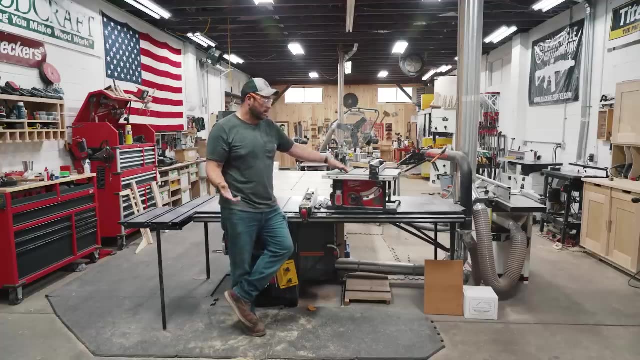 because I think the table saw for woodworking is the most versatile tool in the shop And I think a lot of woodworkers feel the same. So getting into one as quickly as you can in your woodworking is going to help you. There's a lot of phenomenal woodworkers out there who work on literally just. 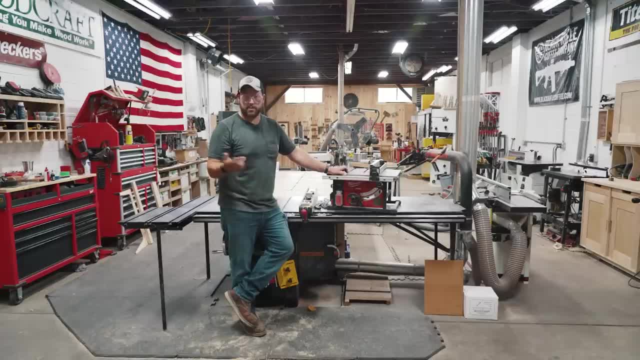 job site saws. My favorite is going to be Tamar from 3x3 Customs. She's had a job site saw forever and she does incredible work, So you don't need this big old beefy guy down here to be good. 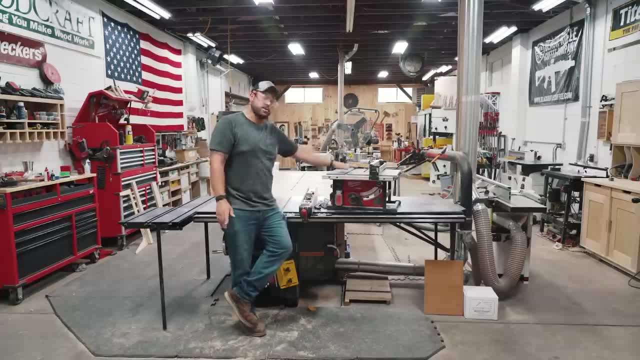 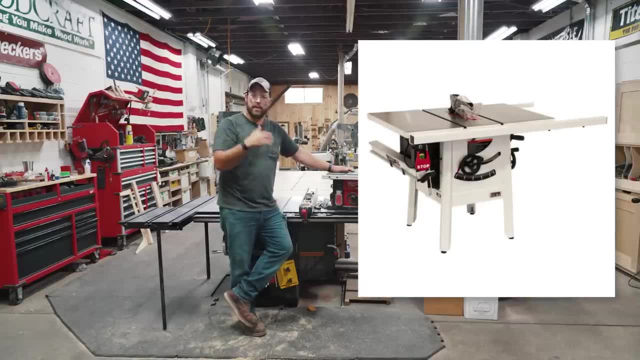 With that, though, there's a lot of options out there, So you've got, like I said, your job site saw. The next level is called a hybrid saw. I used to have one of those in my first shop, If you guys. 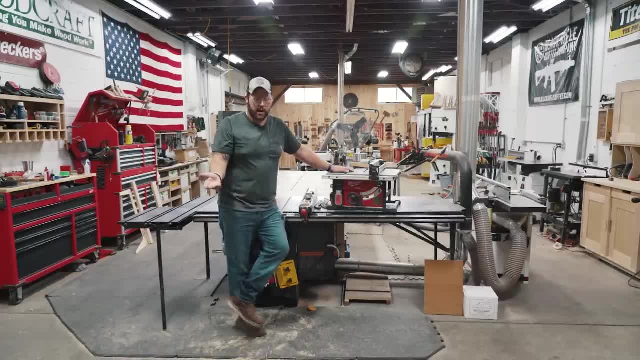 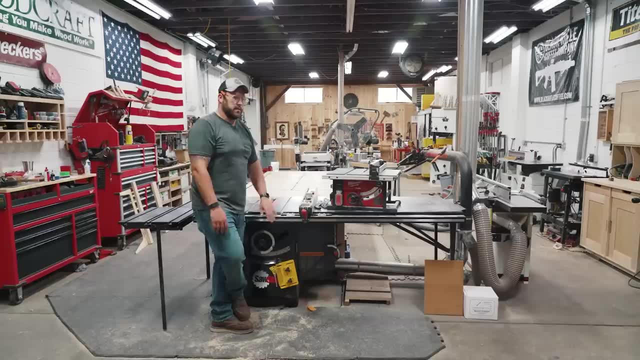 remember that DeWalt saw that I had. that was what you call a hybrid saw, And then you have your cabinet saw, which is what this guy is. This is a five horsepower saw. This is pretty much the last saw I'll probably ever own Going bigger than this after. this is for mostly industrial applications. 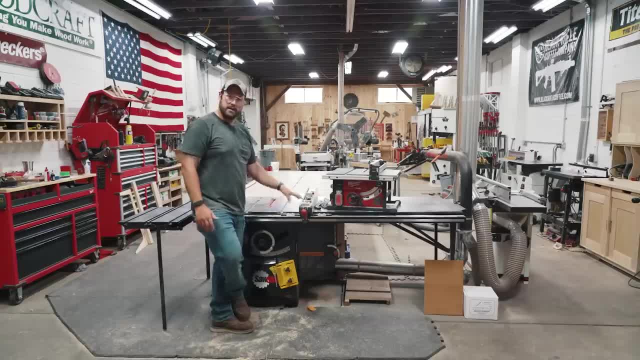 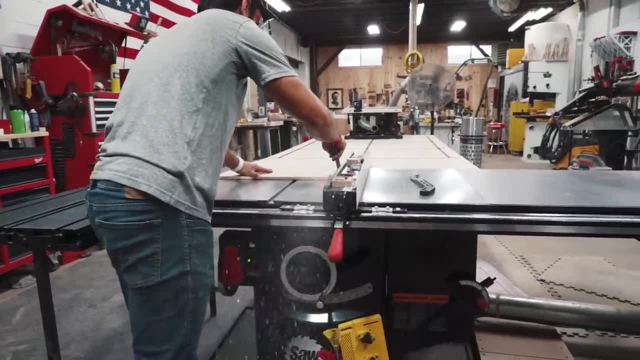 So you don't need to get into a crazy big saw. It is nice to have And it does help. It's going to be the biggest purchase, but also the most versatile thing in your wood shop And something that I highly highly suggest getting into as fast as possible. You're going to 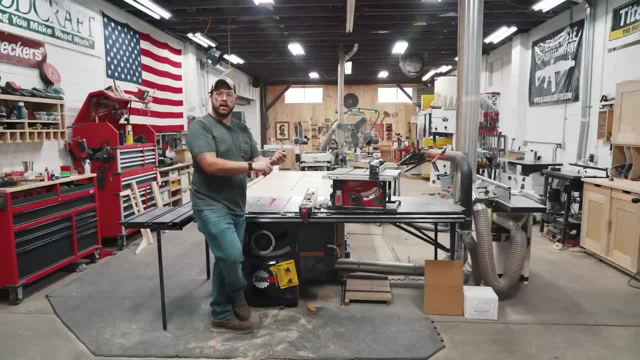 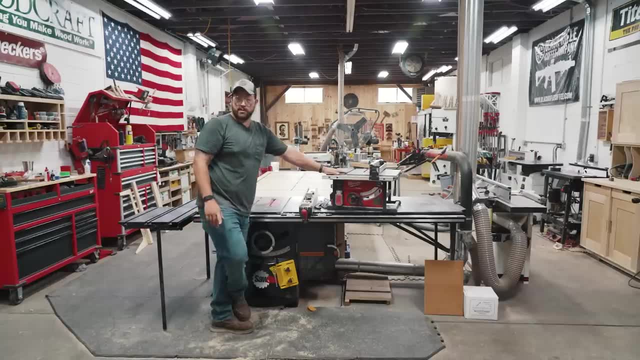 save up for anything, Make sure that it's this. It doesn't need to be a miter saw, It doesn't need to be a joiner. This guy table saw First, big purchase. And if you can't go big first, go with the job. 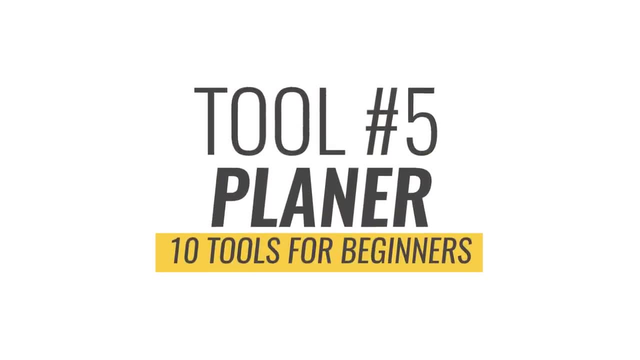 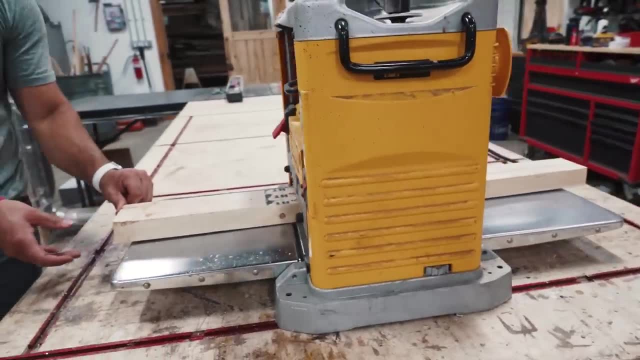 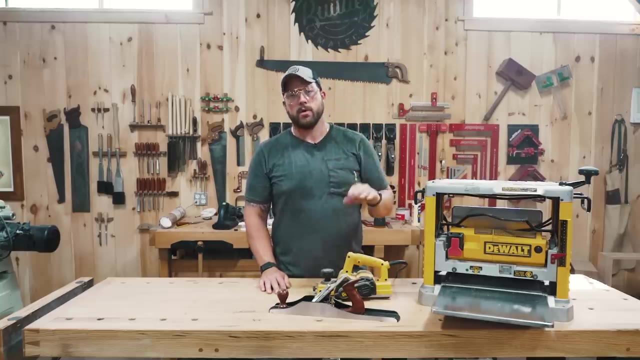 site. You heard The number five tool that I'm going to suggest for the beginner wood shop is going to be the planer. The planer is the tool that makes your stuff, your wood, parallel. It doesn't make it flat, It makes it parallel. You need to understand that. 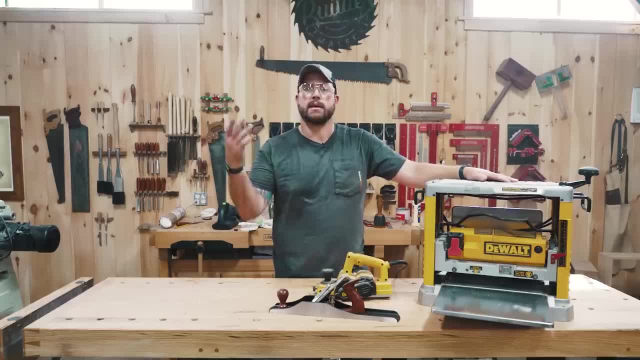 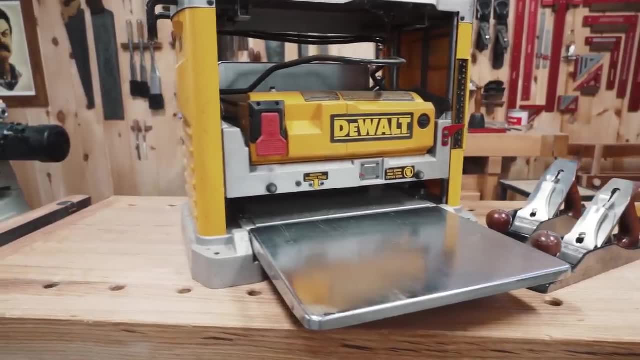 The most important reason for having a planer is because you can thickness materials to your desired thickness. It's incredible. I've had this lunchbox planer- This is a 12 inch- for seven or eight years now. It's the first one I 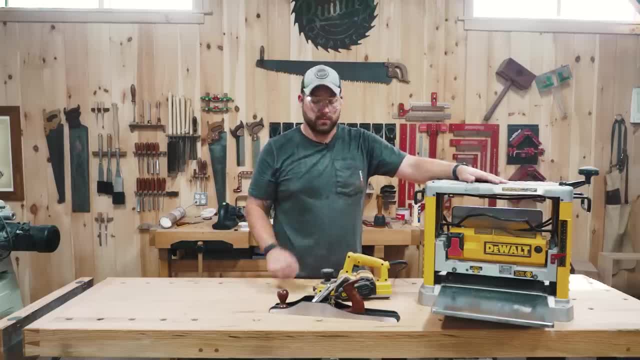 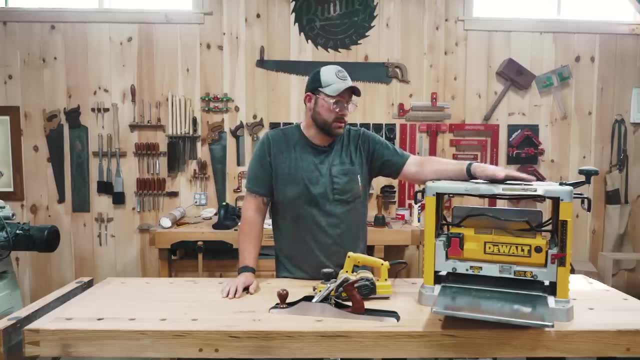 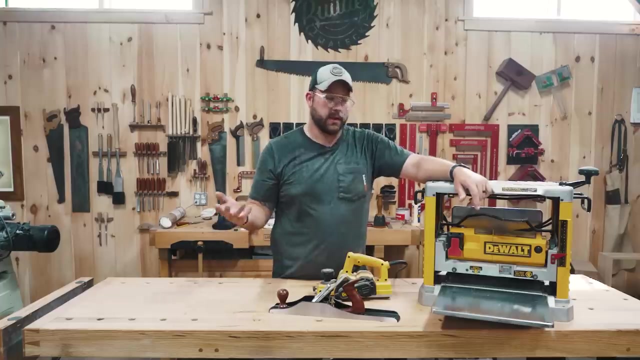 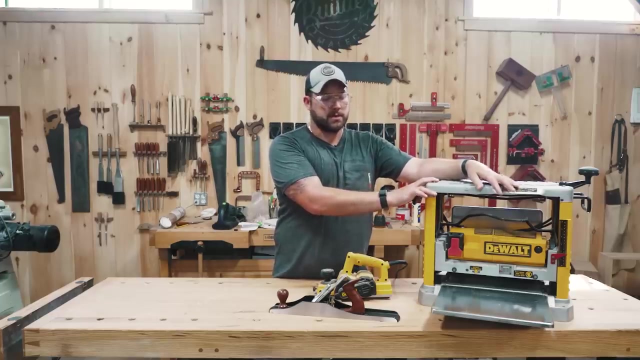 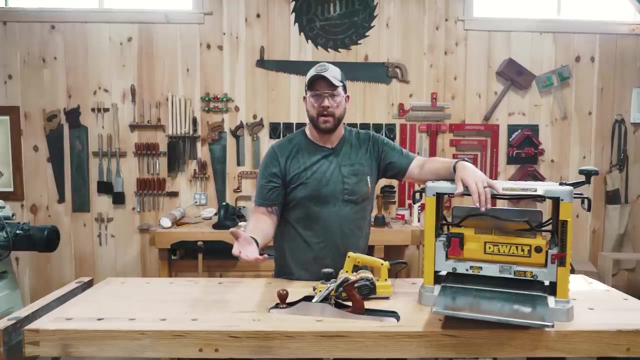 bought. I bought it as absolutely soon as I could in order to basically use materials that were larger and make them smaller. And these things work great. A lot of people get stuck. They start with them. You can also take them to the job site. They do weigh like 80 pounds but they get the job done. They do have their limitations as far as cut capacity, horsepower, And I used to pop the limit on the amount of, I guess, electricity going to this thing all the time when I was using it And I hated that. So other options out, there are just going to be a few other brands. DeWalt also makes a 13 and a half inches. This is really nice. This one has the planer head moves up and down the 13 and a half, I believe. 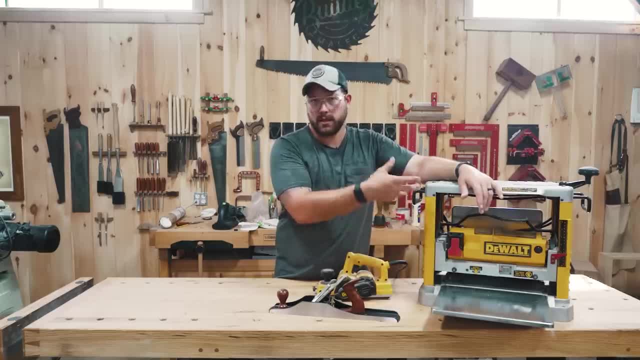 It's the same, except the whole unit is basically the head. They're both really really common. You'll see him a lot throughout a lot of people's stuff. This is what is called an electric hand plane. that can do planing, but it's not a planer. And this is also your traditional hand plane. This is a joiner plane because it's for joining, but it can make sides flat. It's just a long way of going about it in a more traditional sense than you know, just just running it through a machine. I do preface that to use this you do need to buy your lumber with at least one flat side. But it's a really, really common. 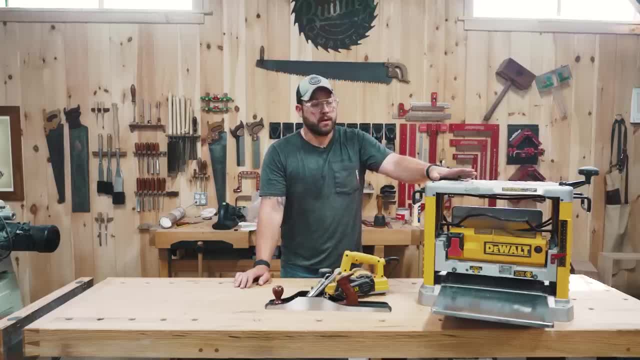 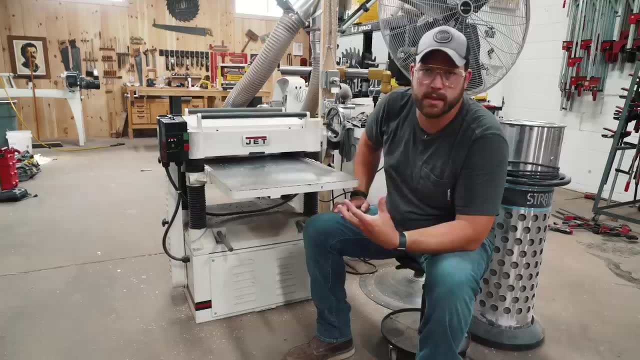 in order to make sure that you're getting things parallel, and then, once you want to upgrade from this little lunch box here, you can come over to what you're used to seeing in my content, which is the 20 inch helical head planer that you guys have been seeing in my stuff for years. this. 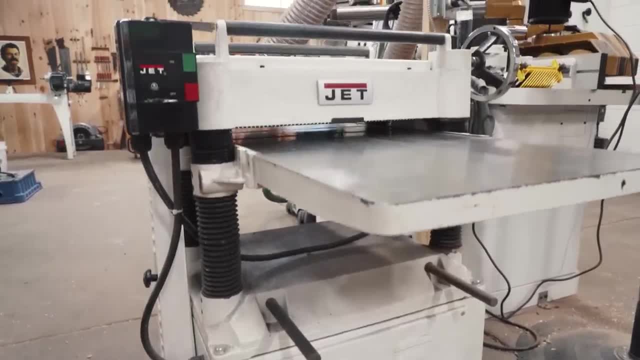 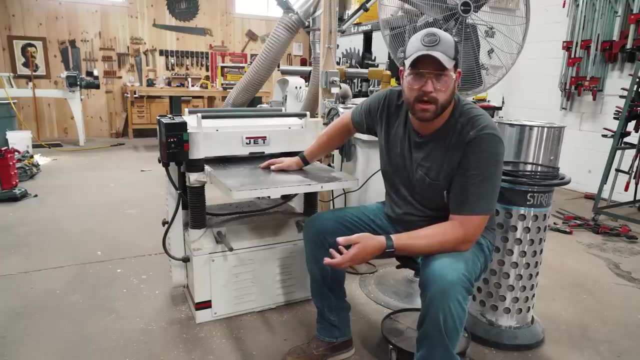 besides, the table saw was the first major upgrade i made to my shop because it increases capacity a ton. the helical head in this thing is amazing. a lot of people will argue that you know, besides the saw, stop. the helical head for joiners and planers is the biggest advancement in woodworking. 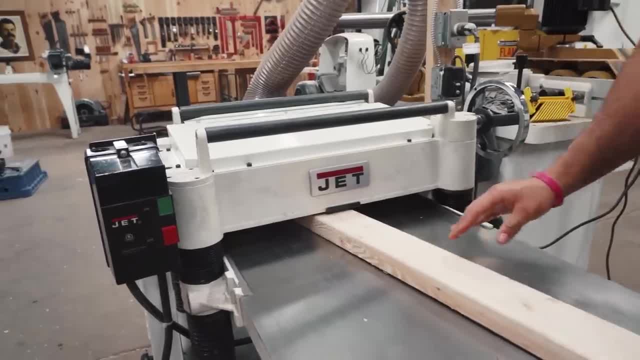 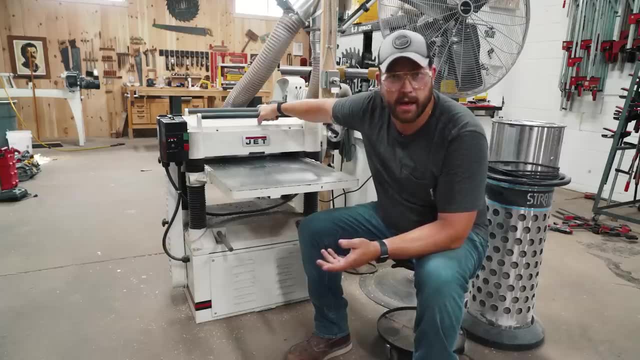 technology that's been like the last like 50 years. a big beefy planer is phenomenal to have, but not a necessity. you can still buy your lumber s4s, but you can get much more affordable stuff that isn't like that, and then thickness it with your planer. so number five: get yourself a planer before we. 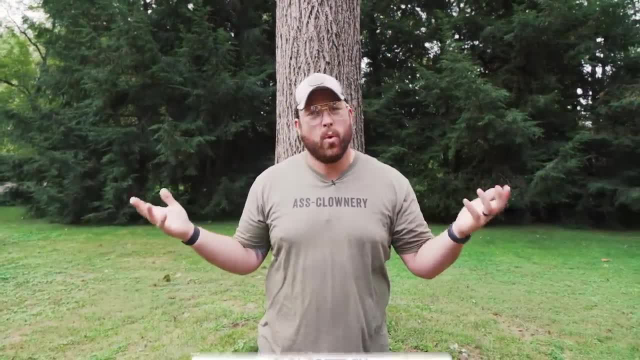 dive into the rest of the tools. i want to thank our sponsor on this video: woodcraft. woodcraft is a huge supporter of my channel and the woodworking community. if you guys are looking to get into the woodworking community, please subscribe to my channel and hit the bell icon so you don't. 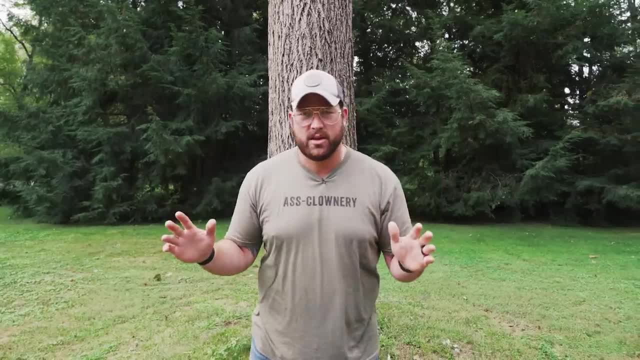 miss any of the next videos and i'll see you guys in the next video. bye, they're gonna have almost everything you need, especially the tools we've got listed here. i've got links down below to everything if you want to check those out as well, but i would 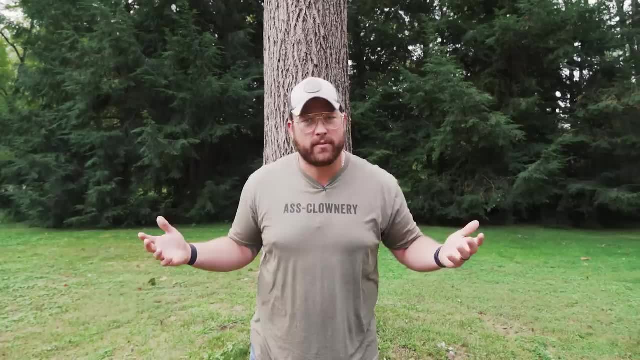 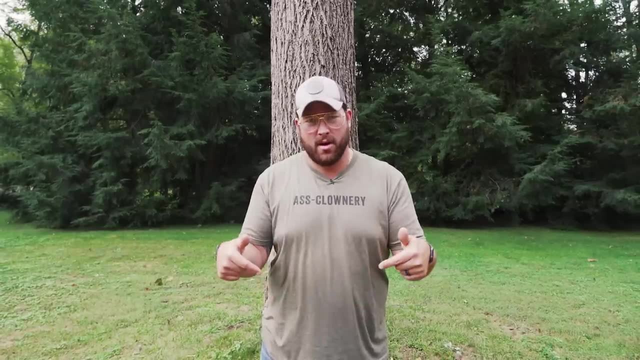 suggest finding a local woodcraft store, getting in there, making friends with whoever's running it and being awesome. we love our store and we know you guys will love yours. check out woodcraft down below and get into the goodness that is woodcraft now. thank you guys for sponsoring. 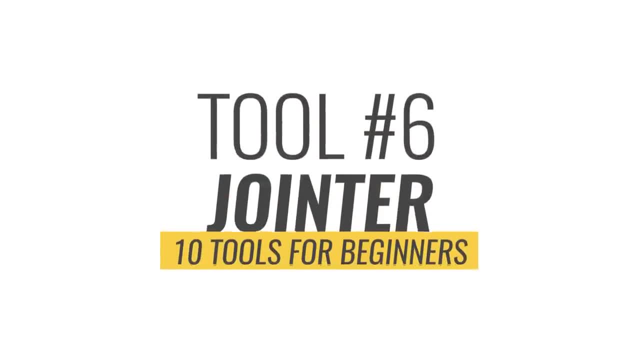 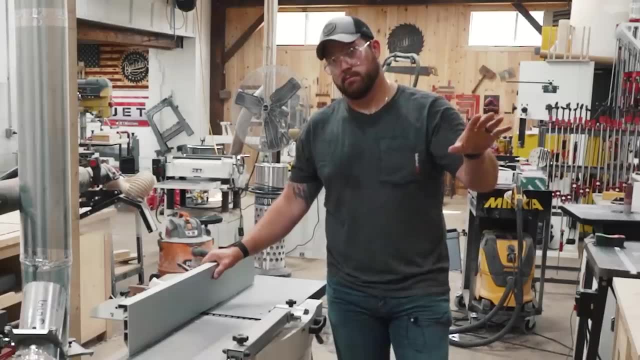 this one and let's get back to the video. all right, the number six tool that you're going to purchase after you have those first five. you got to get those first five first, then you can get into these. that tool is going to be the joiner. 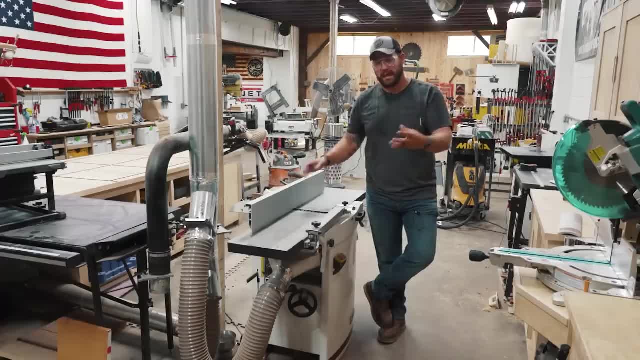 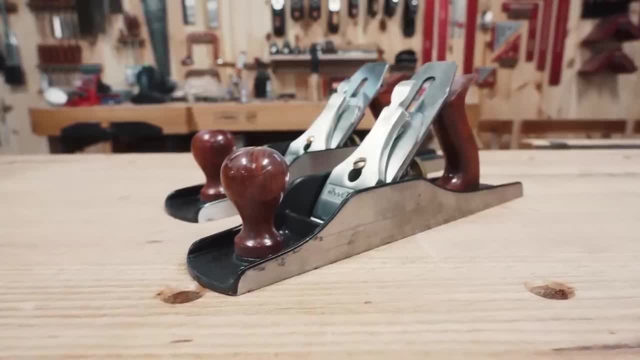 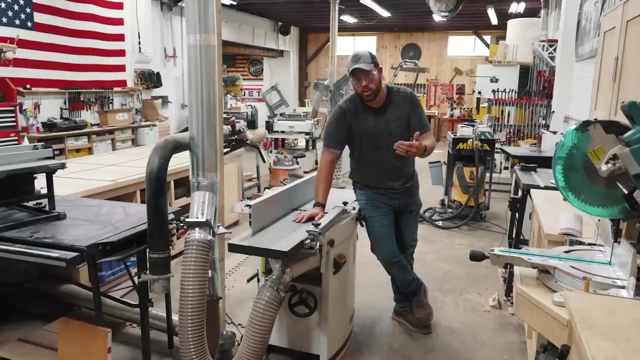 myself. this is my third joiner, and what the joiner does is it creates a flat surface. the reason i have the planer before the joiner is because you can use a hand plane to flatten a surface, which is much cheaper and affordable to get into, and then plane things. you can also purchase wood with. 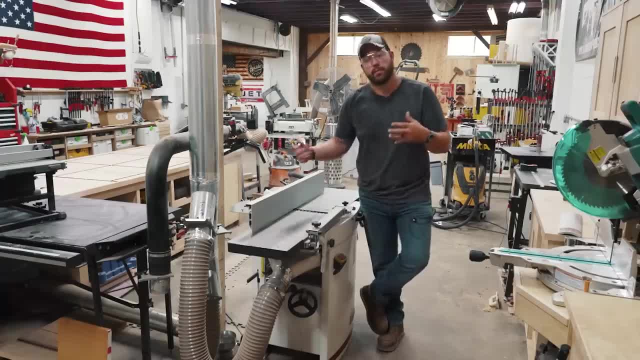 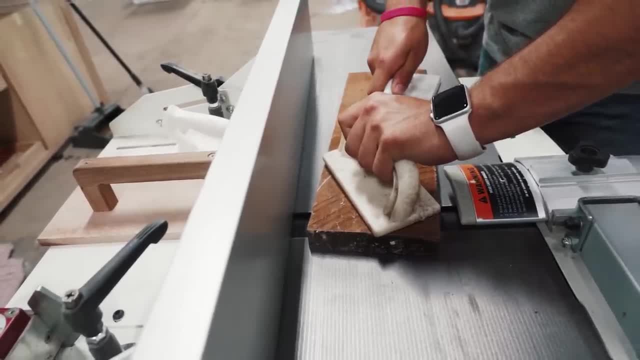 a flat surface and you can also purchase wood with a flat surface. so i'm going to show you how you can get a flat surface or have one surface jointed at your lumber yard to save you money and save you time. the joiner ends up becoming a convenience thing for buying rough lumber for. 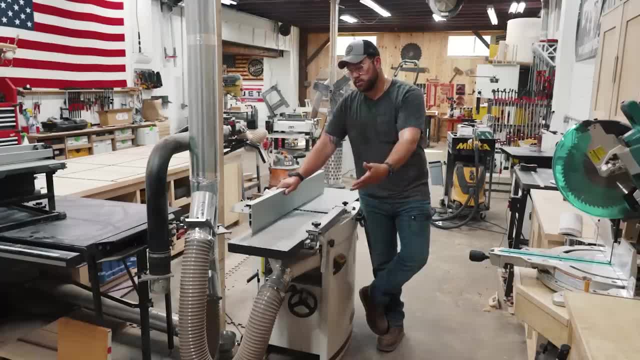 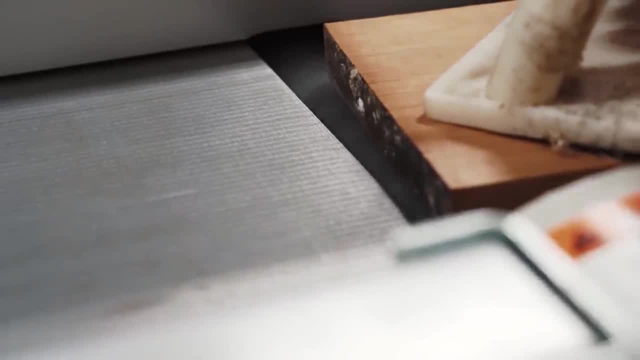 the most part, like i said, creates a flat surface and then you run it through your planer to, you know, make the parallel surface and this also gives you your square edge. like i said, this is my third one. my first one was a six inch joiner that i bought on craigslist. so for all of you out there, 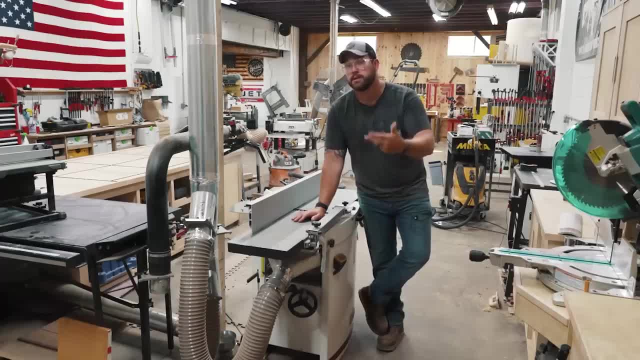 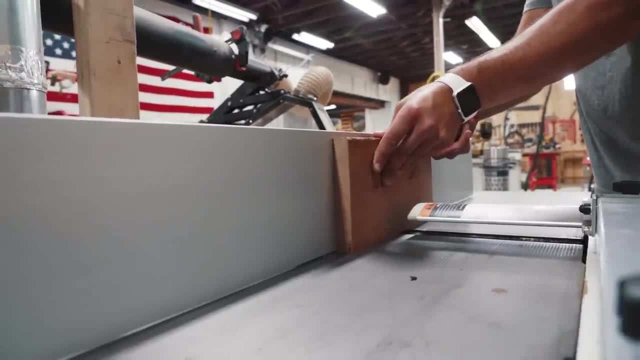 my suggestion is to find the best quality, cheapest six inch joiner you can, and i'm going to show you how you can get the best quality six inch joiner you can on whatever repurposed market there is out there for you. the joiner is a machine that's pretty basic and you can pretty much get a decent quality. 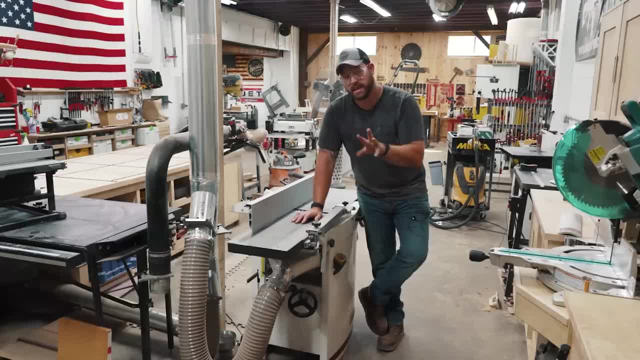 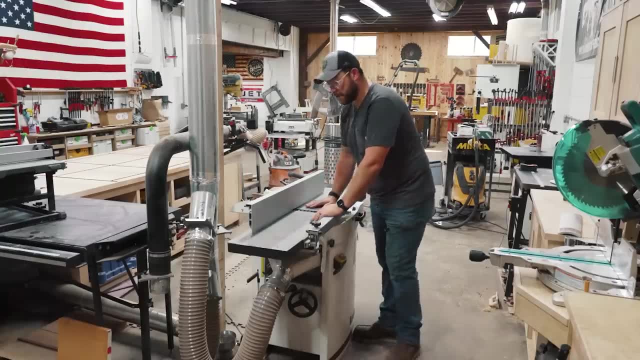 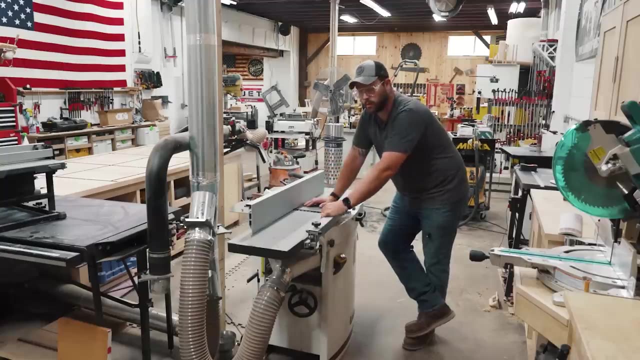 one on the used marketplace when you're getting started. second joiner i had was an eight inch uh powermatic that you guys probably saw a few years ago if you've been watching my stuff, um, and then this is a 12 inch joiner planer combo. we have it for the, the width it's to be able to. 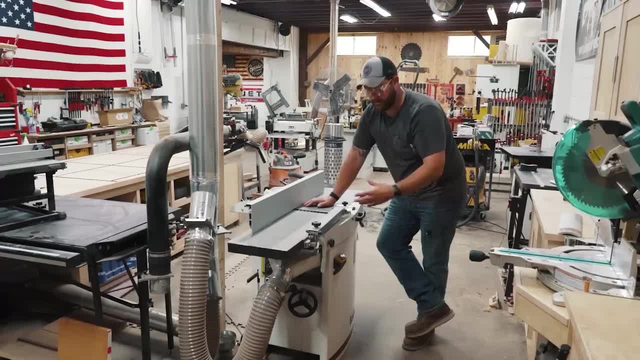 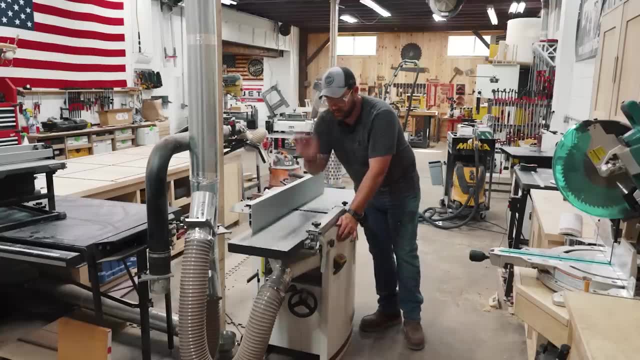 plane our joint wider boards and i highly suggest and also keep in mind, even if you're getting a lot of low quality woodwork to get your joint shorter, you're going to want to get it and they can't afford it. straight knives are not bad. they. 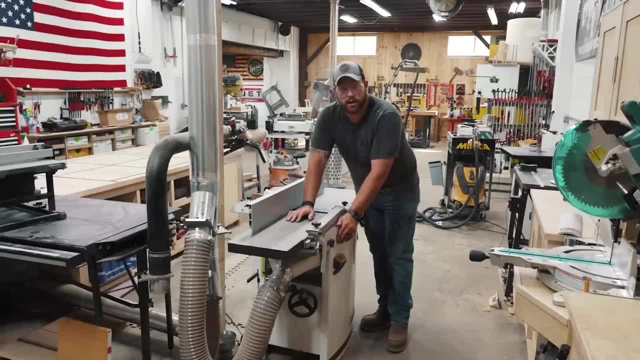 just you got to replace them more often. but the joiner does allow you to square lumber quickly and allows you to buy lumber cheaper, and if that is the route you're trying to go with your woodworking is to get your most affordable raw materials, a joiner is definitely going to be. 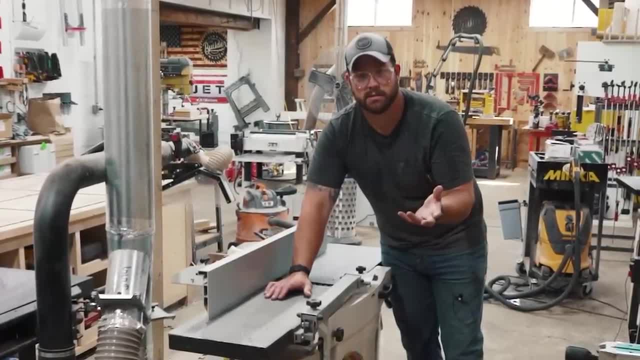 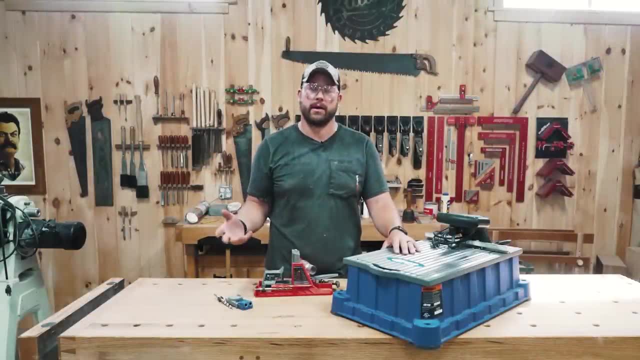 next. but, like i said, i prefer getting a planer first because i already talked about it so i don't need to repeat myself. but yes, joiner number six that i'm going to suggest for the beginner woodworker is going to be the pocket hole jig. 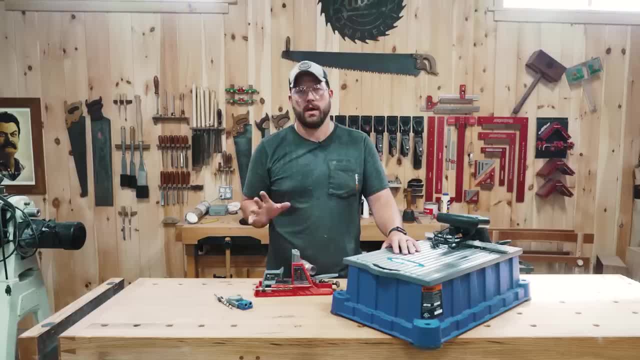 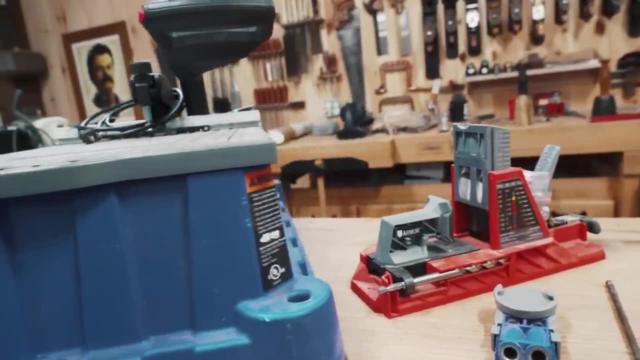 and for all of you out there that think i hate the pocket hole jig, i do, and it's because a lot of people misuse it with that. the pocket hole jig is mostly intended to be used with three-quarter inch material for carcass building, and learning to build cabinets is an extremely important and 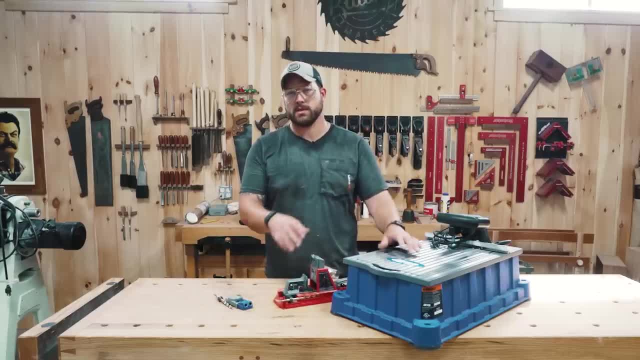 versatile skill set for the woodworker, as much as people use this thing to bang two by fours together to make stuff. i got started doing that. i i'm not going to say i'm not, haven't been there, it's just not what this joinery method was intended to do. i highly advocate for using this. 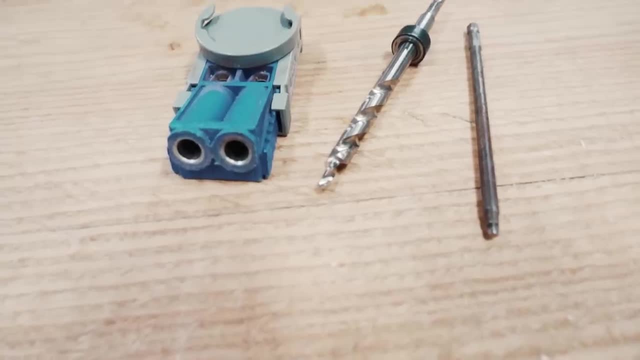 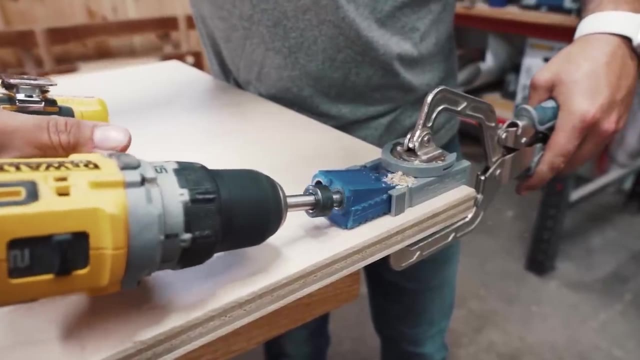 tool properly. there's multiple options out there. the easiest to get into is going to be this little guy. it's called the r3, i think, or used to be. i have like three or four of these and we use them all the time for our carcass building and stuff. armor tools has this really cool jig for pocket. 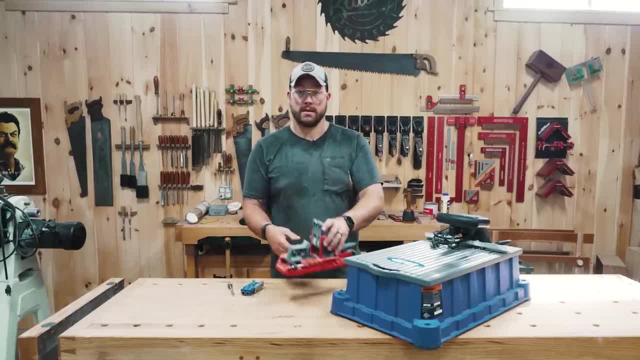 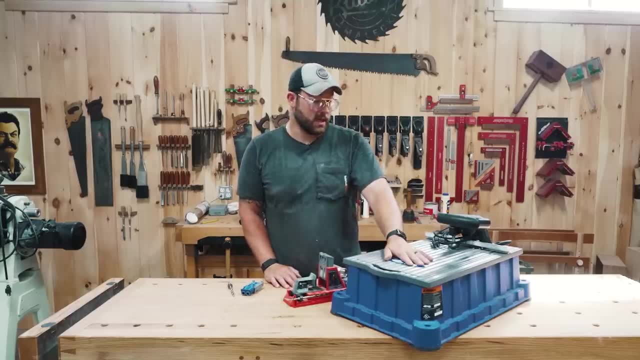 holes. there's a couple companies that make them similar to this. now, craig is like the king of pocket holes and they also have something similar. i think it's our k5 or four or whatever. and then craig also makes this incredibly amazing foreman, which we use for pretty much all of our 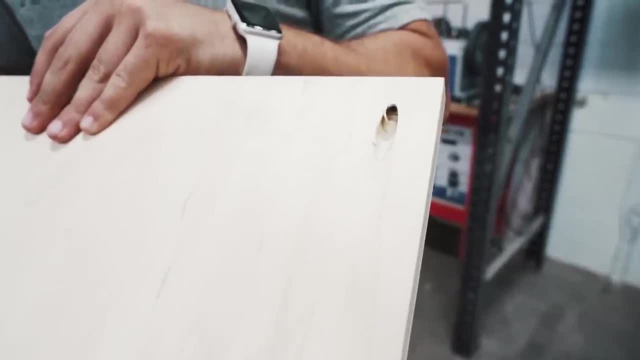 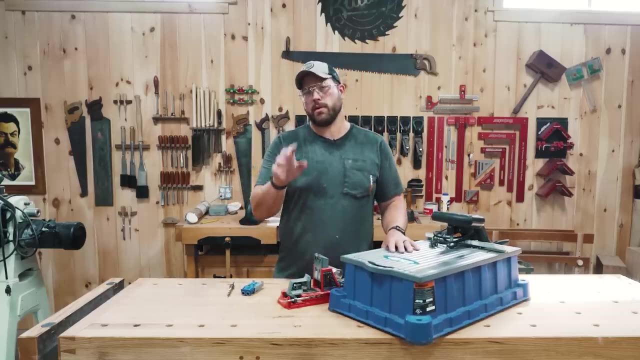 carcass building. but the reason i suggest getting into the pocket hole jig is one, because you can learn to use hidden fasteners, and two, you can pretty much learn to make cabinets. just don't abuse it like. you should not be building farmhouse or trestle style tables with pocket holes, trust me. 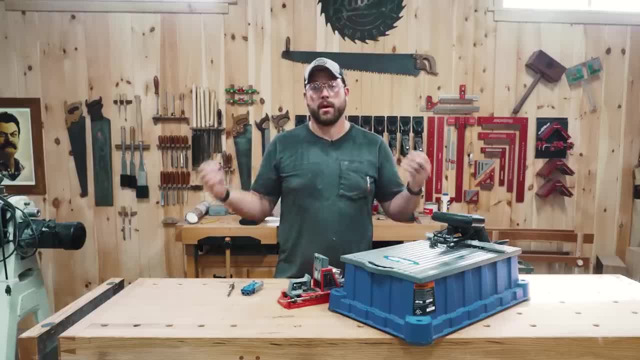 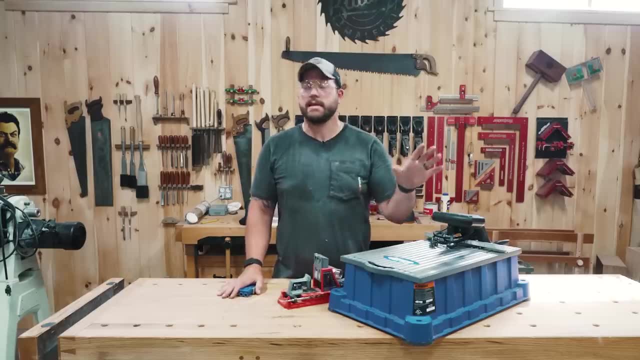 i get enough dms and comments on things exploding apart. if you're not understanding why- and it's because they use pocket hole joinery and not like real joinery- just take the time to learn how to do any type of other joinery for woodworking besides pocket holes and you'll see and you'll understand why. 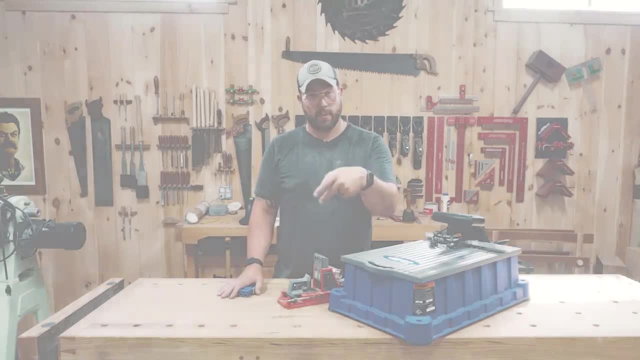 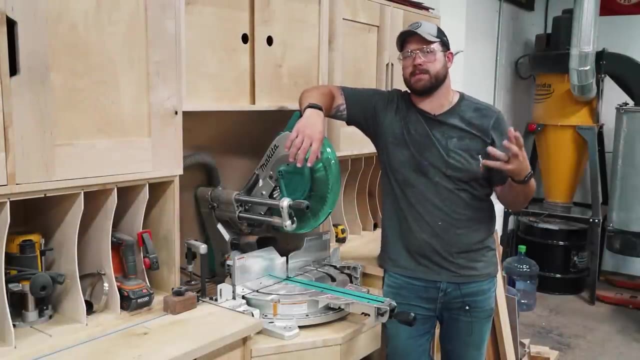 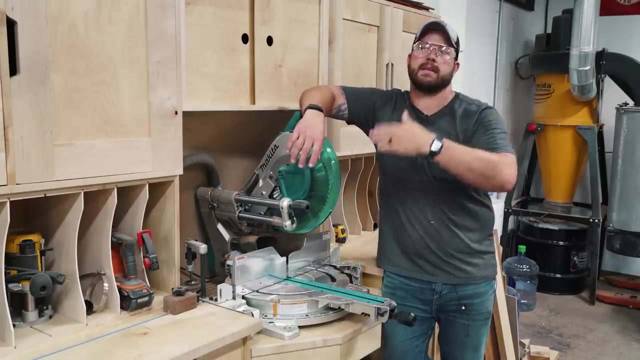 i love them, but i love them being used correctly. number seven: the pocket hole jig. all right, real quick. just to remind you, remember, these are in clusters of five, they're not in a specific order. um, so by saying that this is the number eight, it could actually be six. it doesn't matter, just buy these after you buy the first five in my, in my. 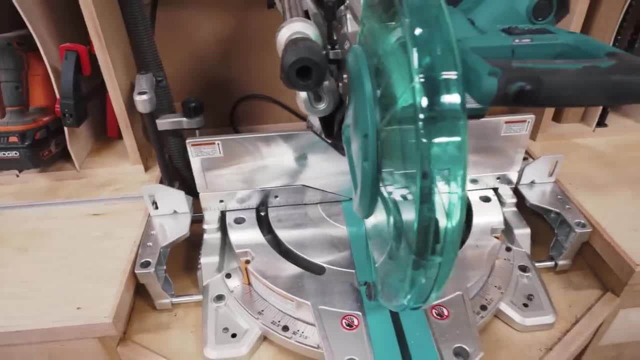 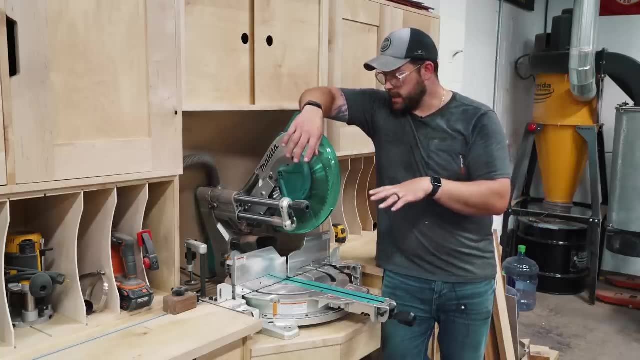 opinion. uh, the number eight tool we've got here is the miter saw. the miter saw is an extremely common saw in pretty much every shop and garage across the country, here in america at least, um, and it's because it's a great tool. we love our miter saw. we use it for rough sawing. i've had a couple of them. 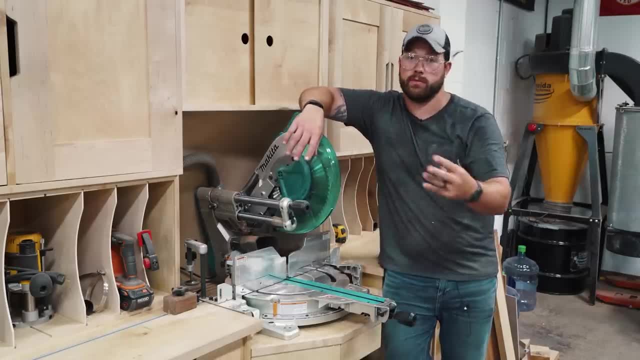 we have a 12 inch to wall. miter saw this is a 12 inch makita. miter saw i have a 12 inch bosch. miter saw you guys want me to do a review with this in the bosch, if you are watching this and you want. 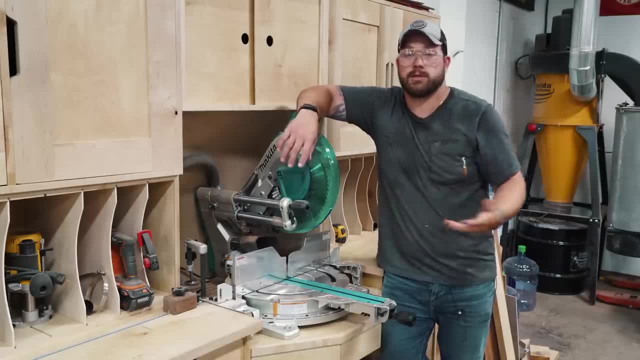 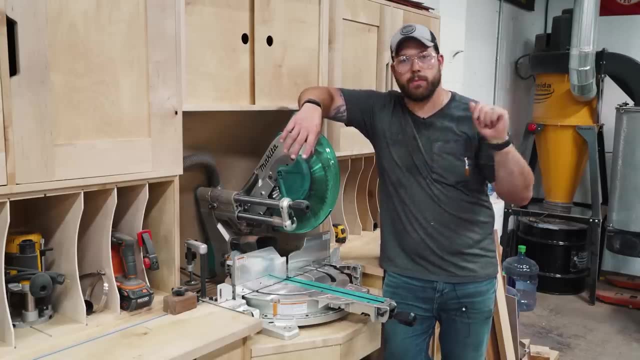 a review. it's not going to happen. buy this one, don't buy the bosch. this has better dust collection, and i'm in a workshop where dust collection matters. there's your answer. all of them cut pretty comparably in the same for my applications. trim carpenters would rip my head off if i said: 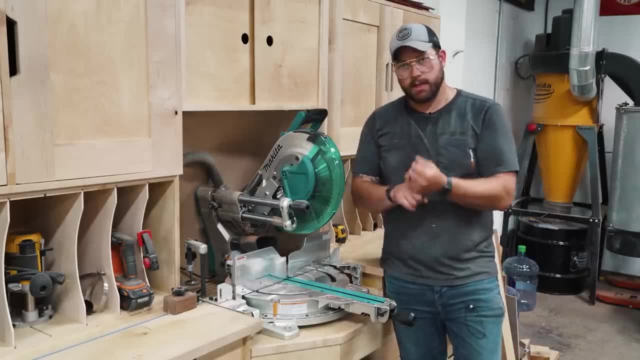 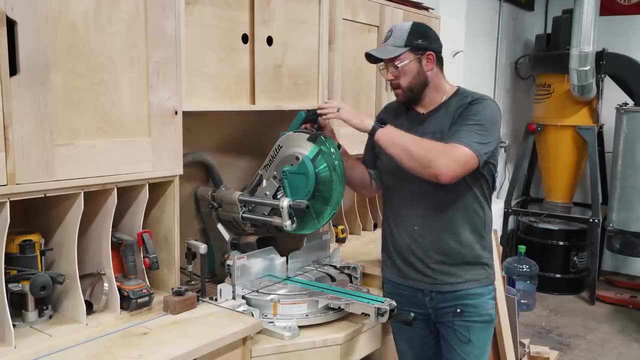 that out loud. so with it you want to be thinking about cut capacity and, uh, the- i guess the- the versatility of the miter itself. here we have a sliding saw, and this is kind of what i'm talking about with versatility. how much distance can you get away from the fence? a fixed 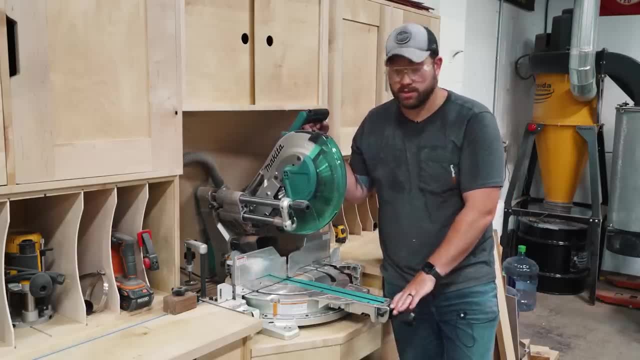 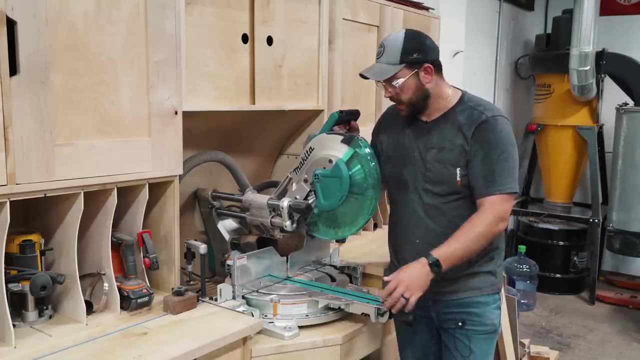 saw isn't going to have as much distance. here i think we can cut up to 13 and a half inches almost, which lets me cut wider boards on a rough saw. i'm here instead of having to do it on a table saw, which saves me time. also, i can think i can do about five inches on the vertical cut with a 12. 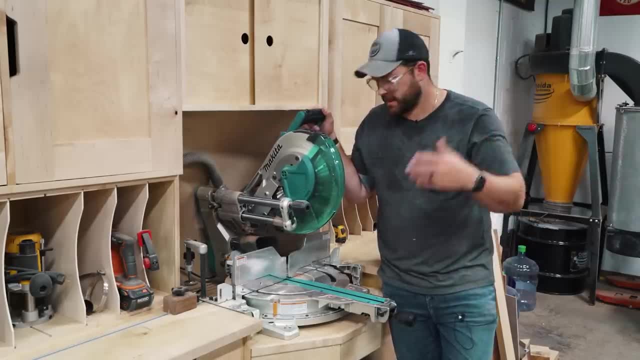 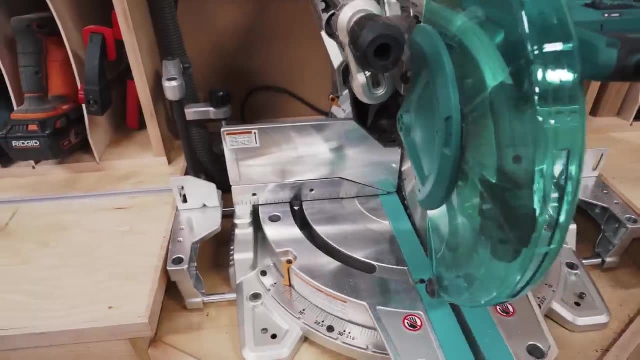 inch saw, a 10 inch saw. you're only going to get about, i think, three or three and a half or something like that. um, so that goes into the equation as well. also is the miter of this saw. specifically, miter is left and right and we also have the miter, miter, miter, miter, miter, miter, miter. 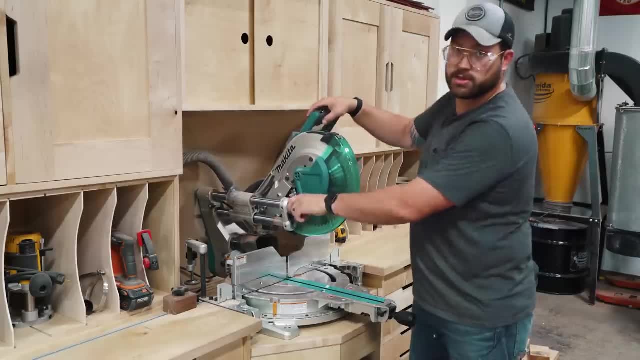 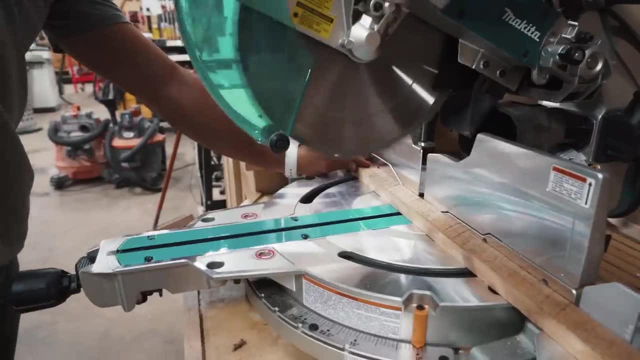 have a beveling on the back side. we never use it in the shop and i'm not going to mess with it because we have this thing square, but that lets you tilt left and right. all that stuff matters for some people. for our shop we're cutting things square, or at miters we don't really. 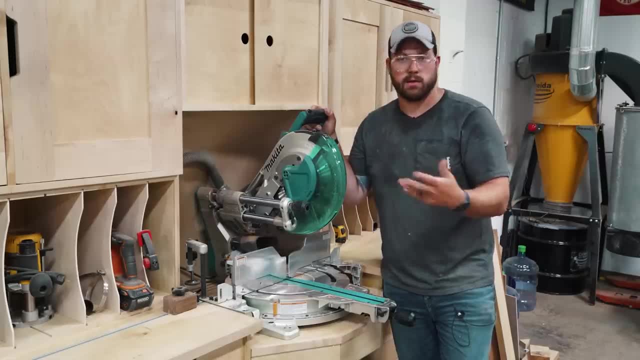 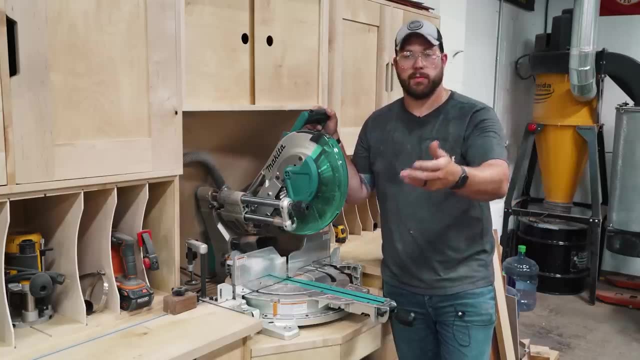 need to use the bevel. so a 12 inch saw, sliding or gliding, uh, works really well for us and in most wood shops i would assume the same and it's going to be my suggestion for your number eight tool, because it's going to help you with cutting things down quickly and, if you set it up properly, 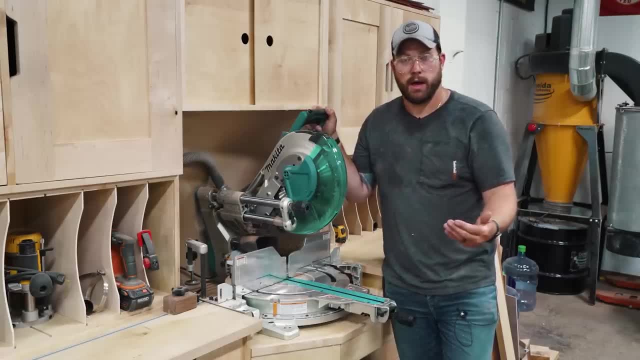 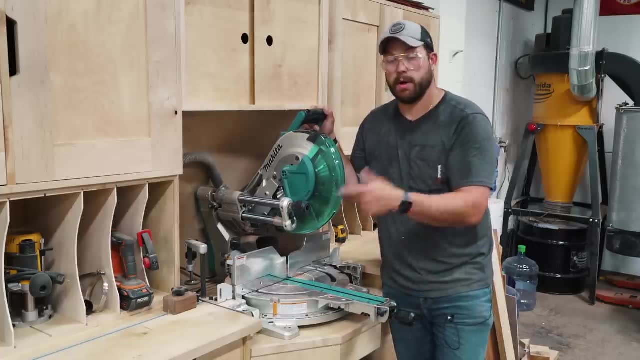 you can actually cut things to final length on it as well. i know a bunch of guys that do that and it works really great for them, so look into them. tons of options out there i'm not going to dive into, but the miter saw number eight, all right tool number nine and i'm going to get a lot of pushback. 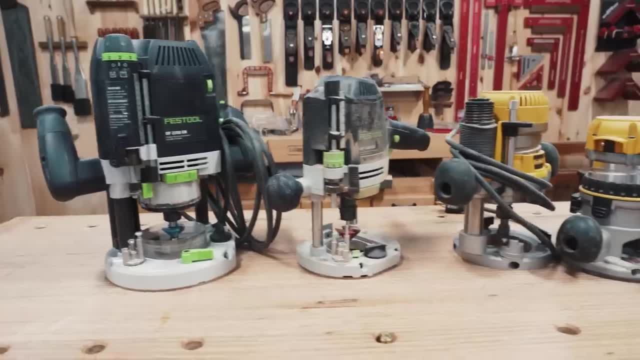 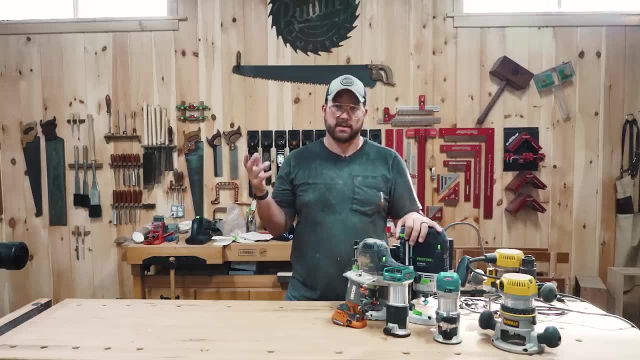 on this one from woodworkers is the router. the reason i have the router kind of this low on the list is because it's a terrifying tool. it really is. there's a cutter head spinning at thousands of rpms in your hand and you're going to want to make sure that you're going to be able to cut it. 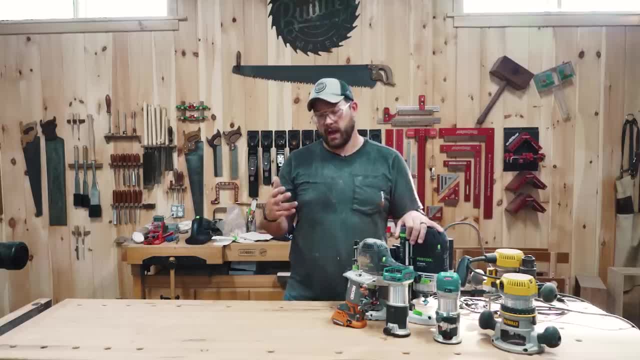 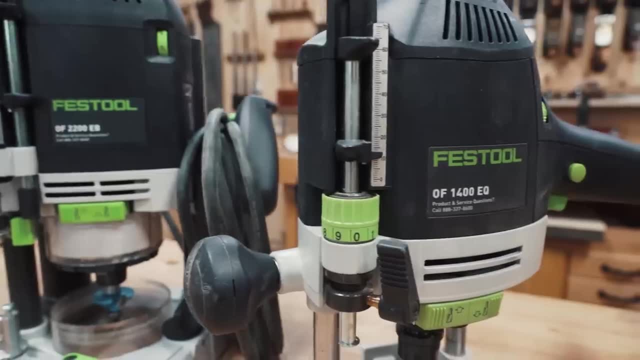 and it can be scary. it's the reason i have it down the list is because i i advocate for becoming comfortable within the wood shop before getting into a router, but, that being said, the router is probably the most versatile tool in your shop. you could do the most with one of these um compared to 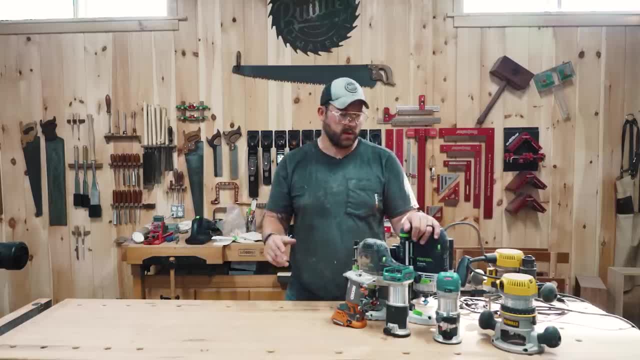 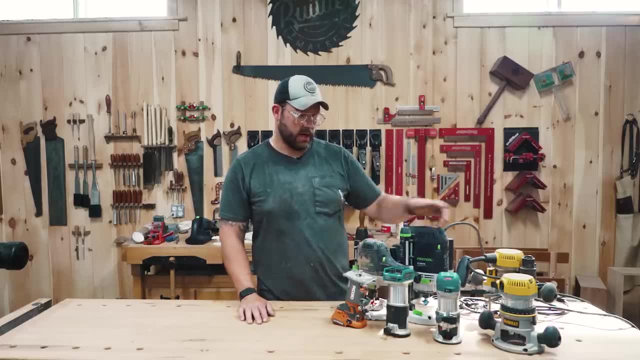 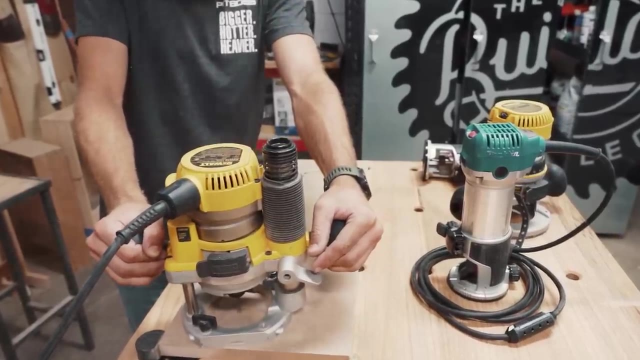 what you can do with everything else besides. maybe the table saw that's arguable. but, um, we have a, a ton of routers. um, here we've got what is that? six, seven, i can't count- seven, seven routers, and i think i have four more throughout the shop and we use them for a ton of different things. you know, we have big, beefy ones. 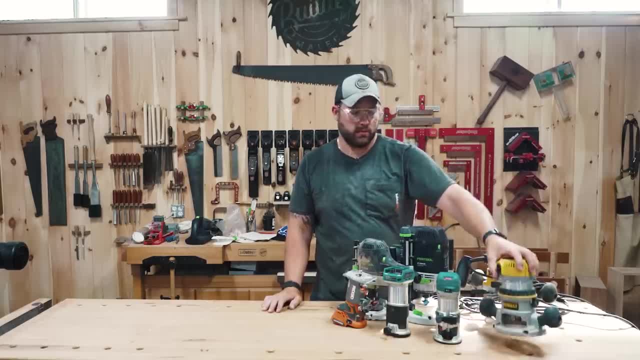 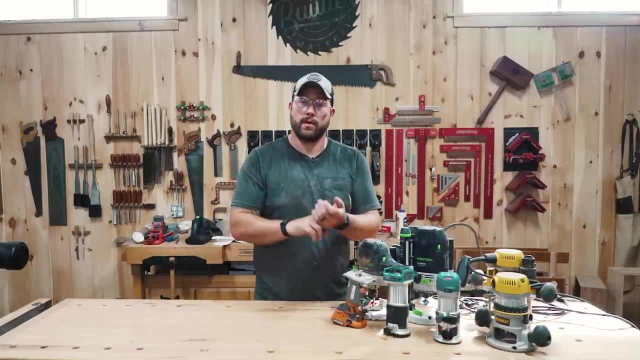 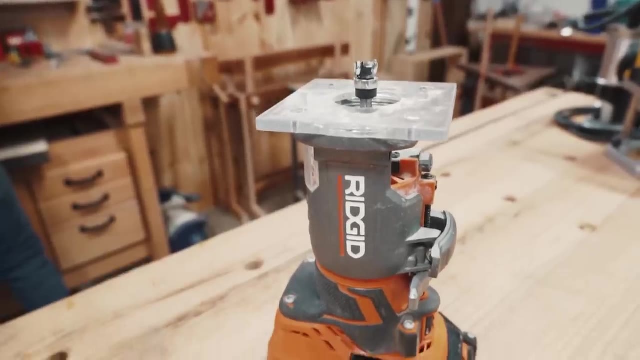 for flattening. we have just general- uh, you know, regular- i think that's a three-quarter horsepower routers that we have dedicated heads in them. whether it's a chamfering bit, whether it's a flush cutting bit, i keep a dedicated bit for templating in this guy for cutting dovetails. 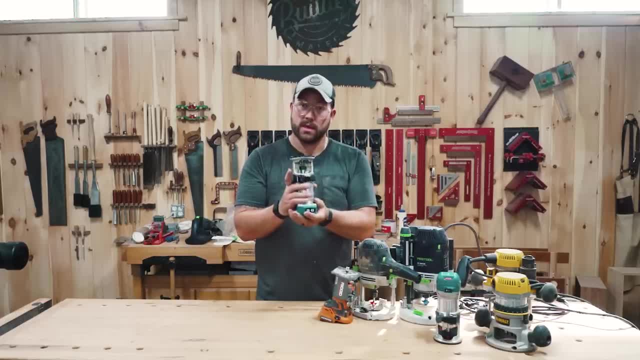 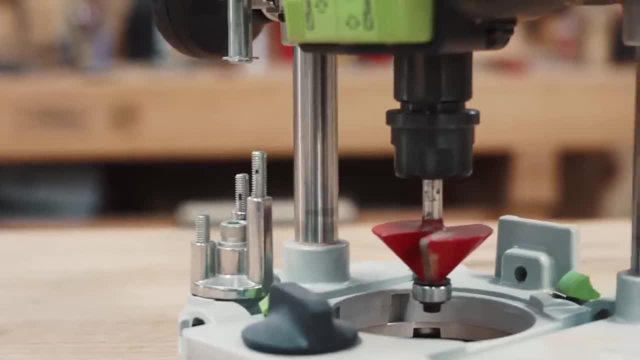 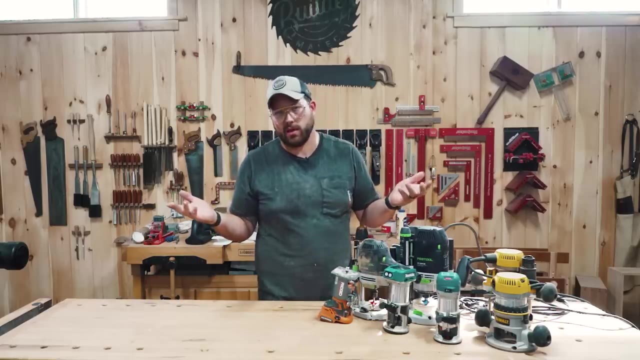 we keep a dedicated bit in the cnc shop in a cordless palm router for cutting tabs on things out of cnc, so you can easily see, uh, how having a bunch of them can become in handy. but with that it's because they're so versatile. you can cut almost almost literally anything. 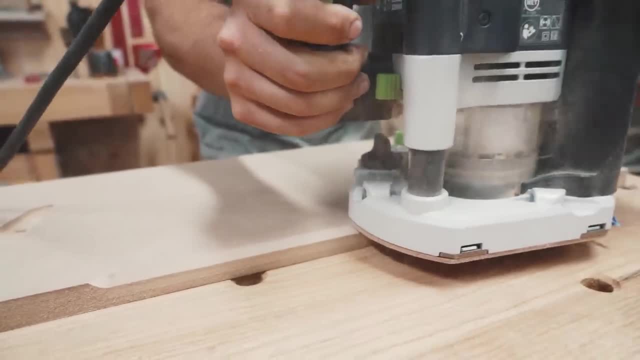 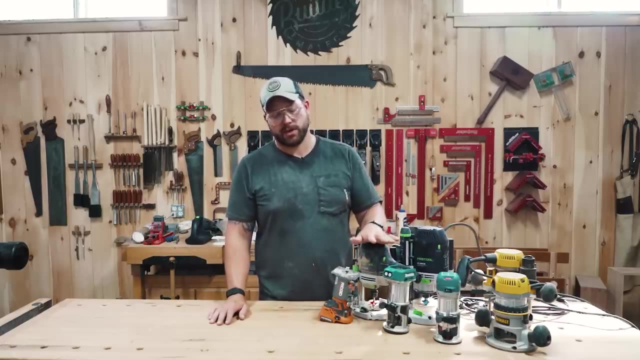 you want, whether it's joinery, whether you're doing flattening, whether you're trying to cut straight edges, and that's because there's so many different bits out there. the router is definitely a tool you need to have in your shop. you just want to make sure that you are being safe and you're. 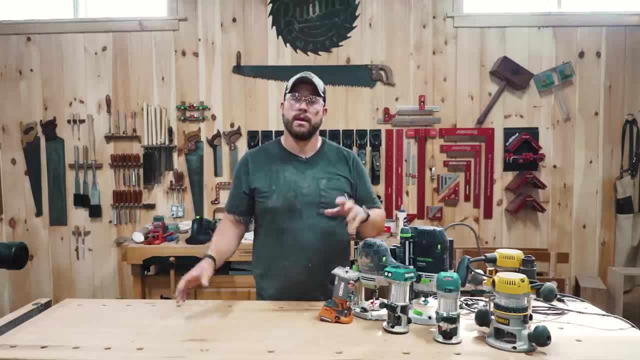 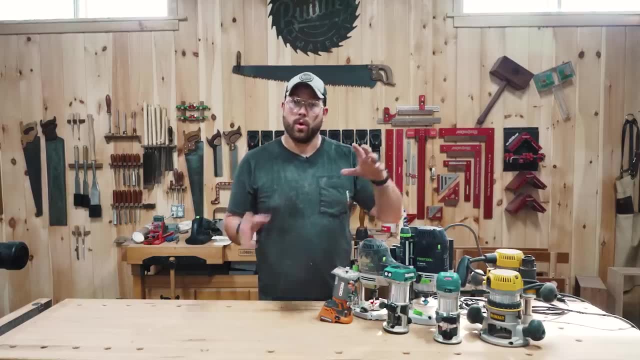 being careful. the last thing i'm going to suggest, if you're getting into buying one, is keep your eye on your effects the whole time your block is going to be took balance out. i would typically snag up guys like this in pairs during the holidays sometimes, or in bundles with other tools. 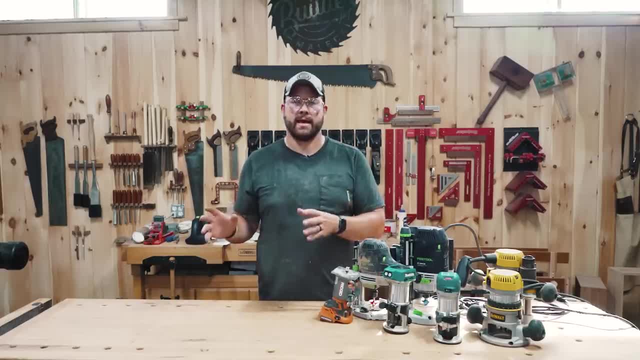 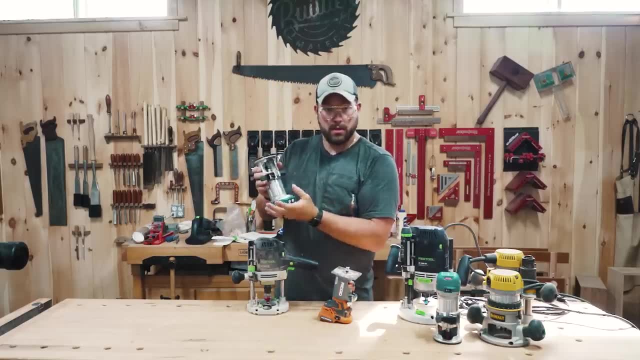 um, they become super affordable. and my last suggestion is going to be for woodworking: try and get a plunge router base and a fixed router base. you have the plunge and you've got it fixed. this is a palm router. this is kind of a standard router and the handles and everything um get into. 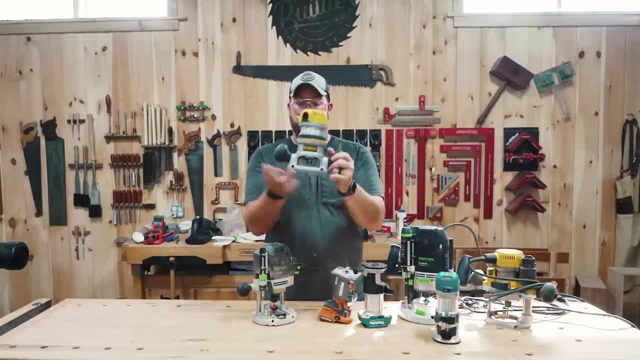 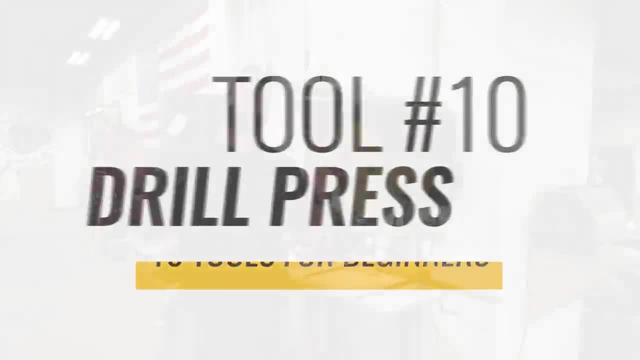 it, but i would suggest these routers. 5,500 Here, your standard three-quarter horsepower. This is a fixed-base, This is your plunge base. Get her done. All right, and the last tool I think you should have in a beginner wood shop is a drill press. 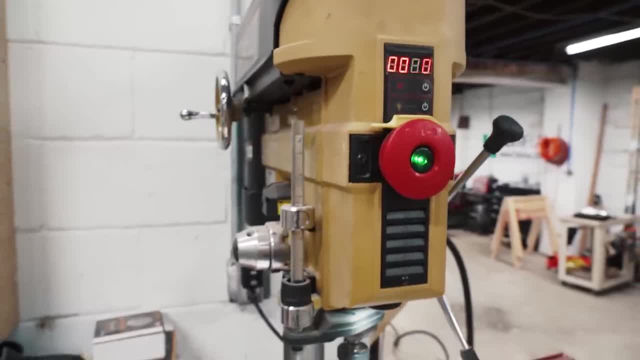 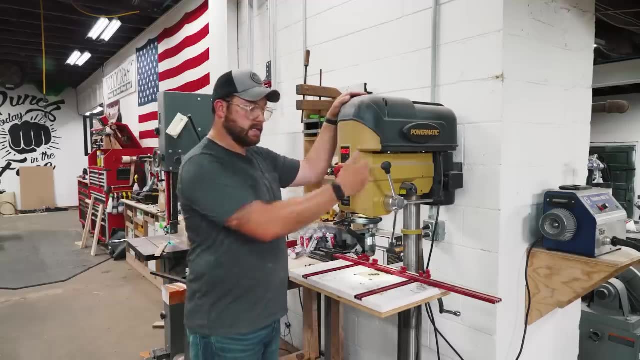 Reason being is similar to the jointer. you can find them very affordable in the used marketplace and they do have a lot of versatility. A drill press is gonna give you an opportunity to create nice, clean, straight holes, which, if you're using exposed fasteners. 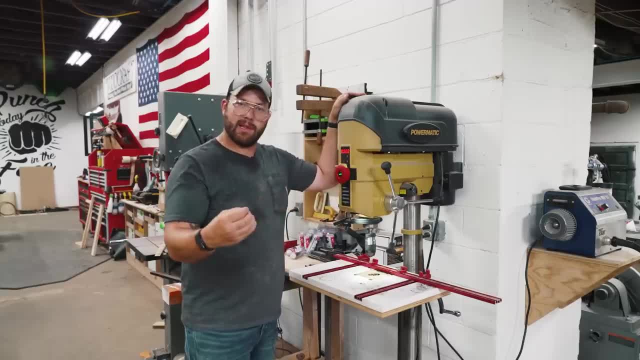 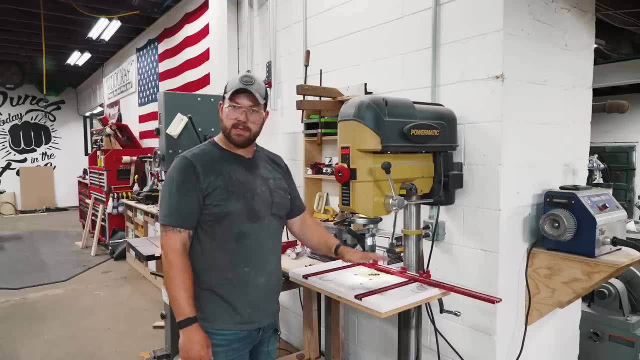 in any type of your woodworking. you can at least make them look clean and you can make sure the holes are perfectly perpendicular to whatever you're cutting. But it also is- it's just one of those staples that, when you need it, you're glad you have it. 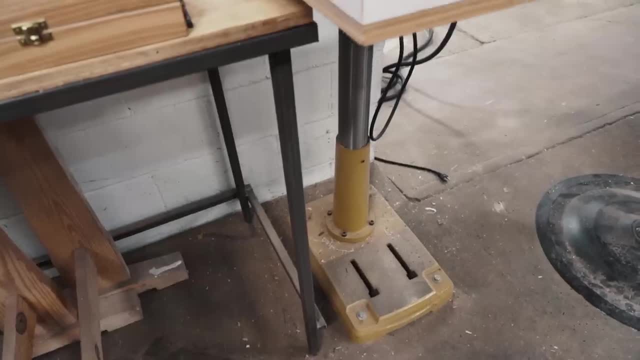 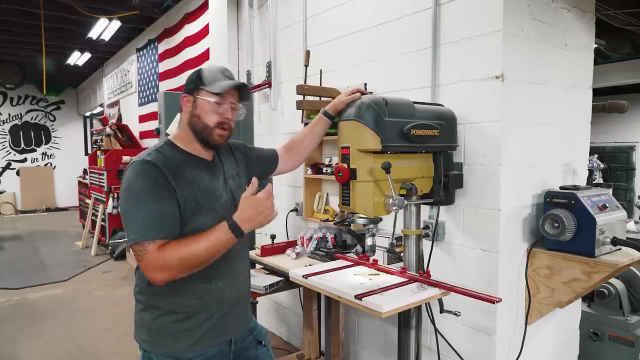 and one of those things that when you don't have one, you drastically miss it. I upgraded to this floor model a few years ago and this thing's a monster. I'll probably never have anything bigger than this, And we use it a ton. 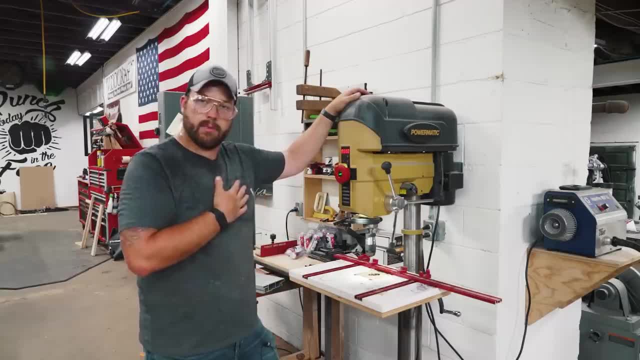 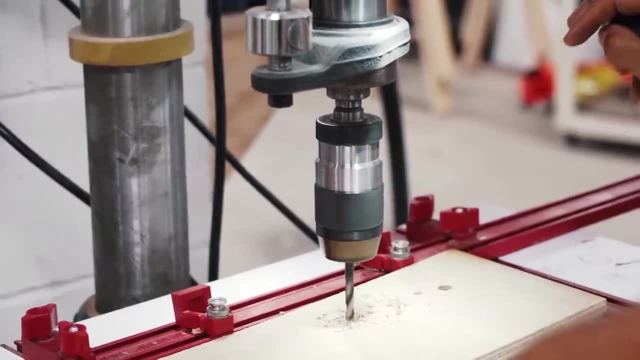 For a lot of stuff, Mostly in our shop is going to be cutting holes specifically in places that we want them, because you can use a fence on a table and you can set up stops and guides for repeatable plunging action with the cutter. 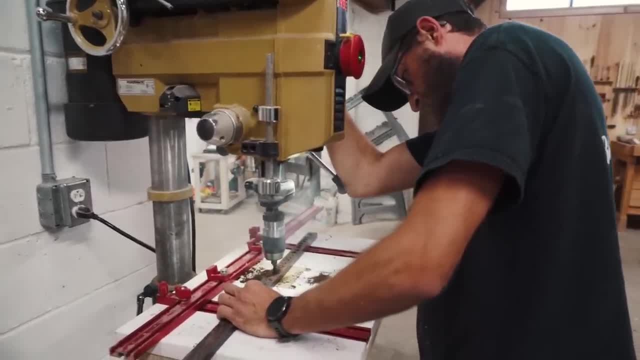 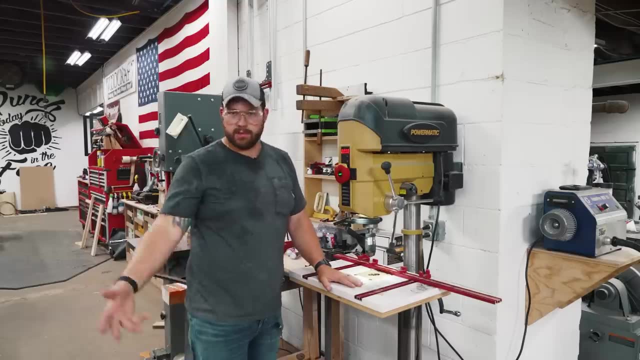 as well as we have a plug cutter bits that we use to fill holes and stuff in a lot of the furniture. if we're using a face screw or something that we wanna look pretty, You're definitely gonna wanna use the drill press in order to do that. 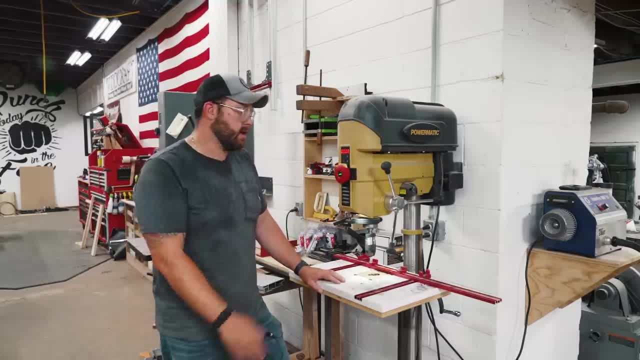 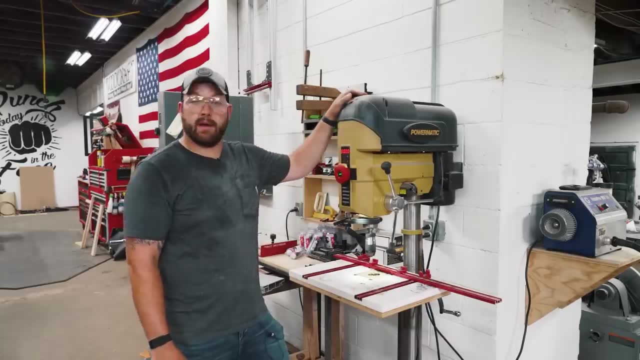 Bench, top or floor. you're in a good place if you have a drill press in your shop. You've got a lot of things that you're gonna find use for it with. I've had one since the minute I found a good price on one. 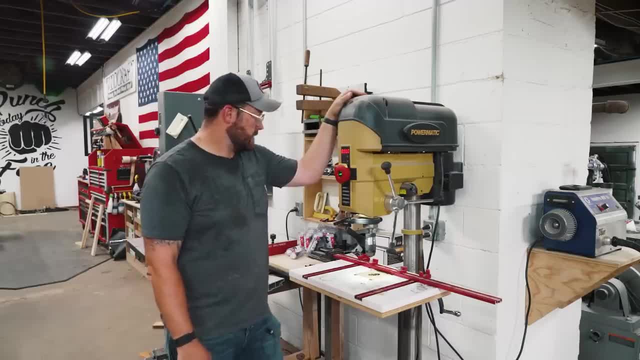 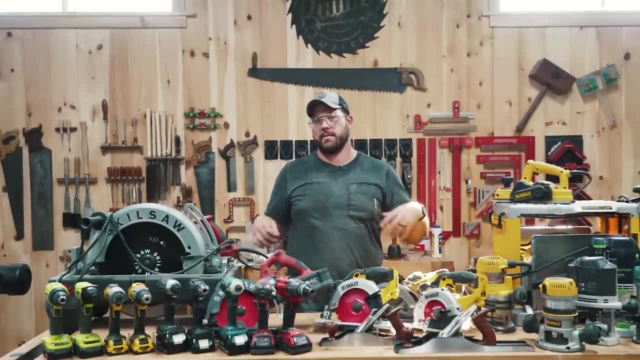 I used to have a bench top model and after I upgraded to this I doubt I'll ever get rid of it. So number 10, the drill press, And that's gonna be a wrap on this one. I understand it can be intimidating. 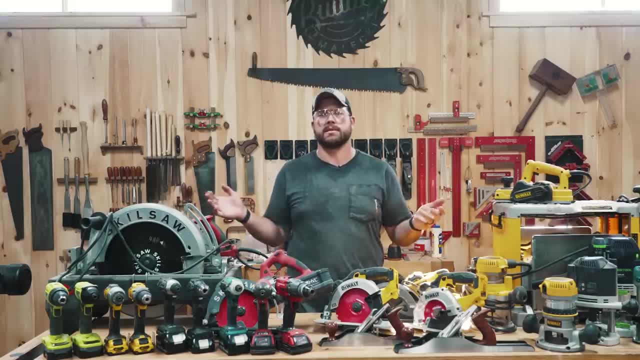 to get into woodworking and confusing, but hopefully this cleared some things up for you guys. I have links down below to all kinds of tools that I suggest and I use if you're interested. Also, if you wanna support the channel, buy some damn merch. 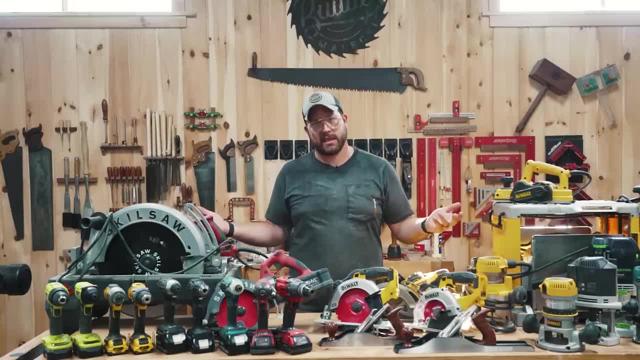 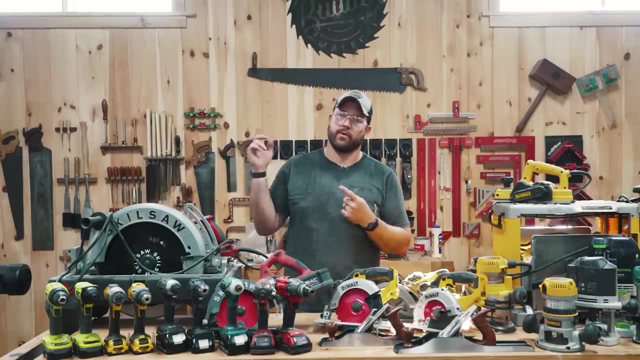 We're working hard on it and we know you guys are loving it. And, lastly, I genuinely do really appreciate each and every one of you for tuning in, And if you wanna see another tips video, I've got it linked up for you right here. and I'll catch you over there. 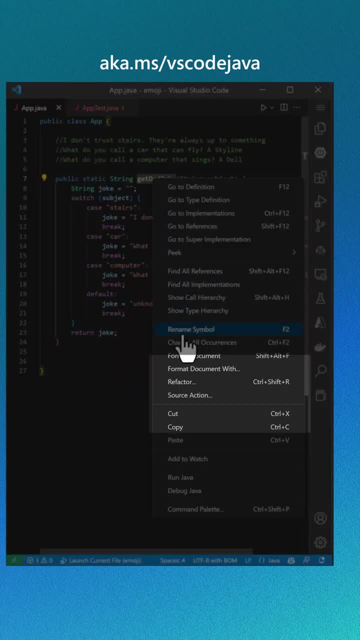 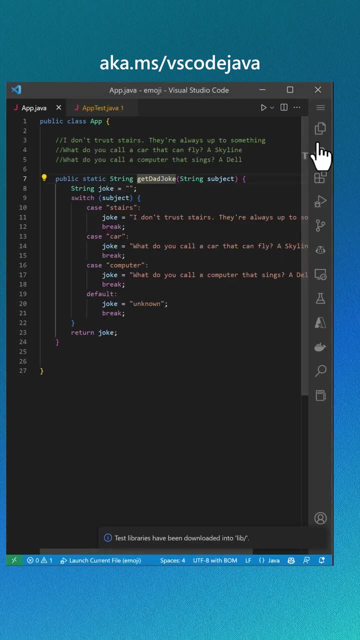 Java testing in VS Code is super easy. Start your testing by selecting source action and then generate tests. It'll add the libraries necessary for your test framework. We're going to choose JUnit and you can see there, I've got my libraries. Now select your test file and 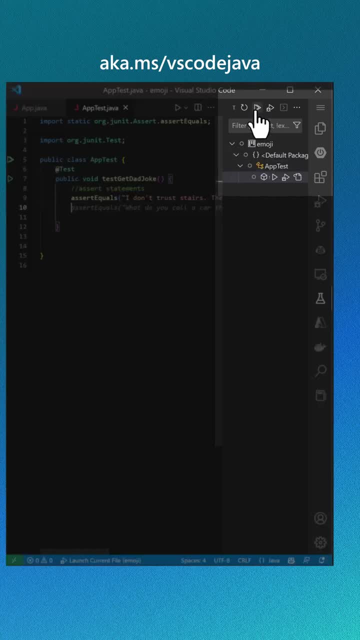 let's ask Copilot to create our test for us Run your tests, and it's easy as one two dad joke.